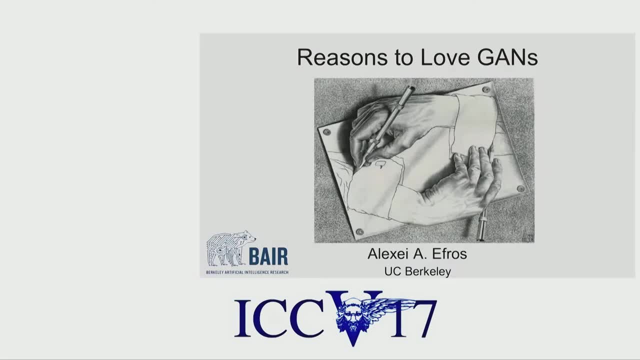 Thank you for staying around until the end. Since I'm the last speaker and we had some wonderful but quite technical talk before me, I thought I would wax poetic and then show you some pictures so that you don't have to really work too hard for this talk. 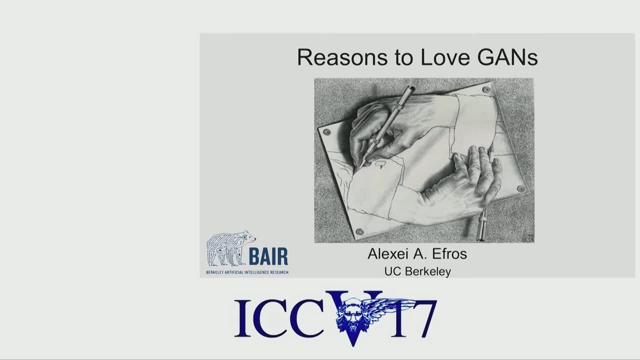 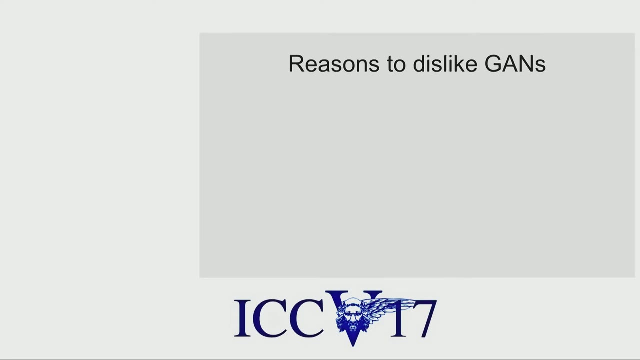 So I thought I would change my title a little bit to the reasons to love GANs, because this is really like a love fest to Ian and the wonderful work that he has done. But before that, of course, you know, have to have some disclaimers. What are the reasons to dislike GANs? And I think some have just been mentioned. 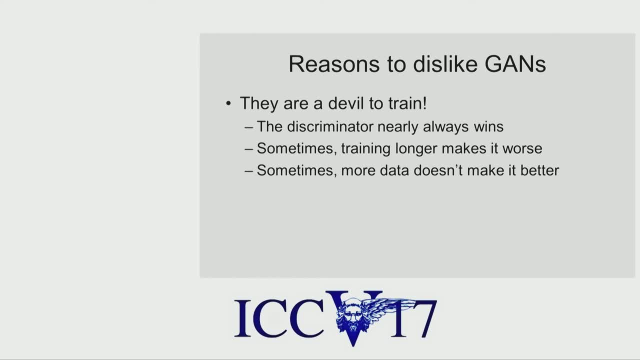 They're a devil to train and you know some of the issues people have already mentioned. You know the discriminator nearly always wins. Sometimes training longer makes it worse, Very annoying. Sometimes more data doesn't make it better, which is I don't understand how quite it is how it is. 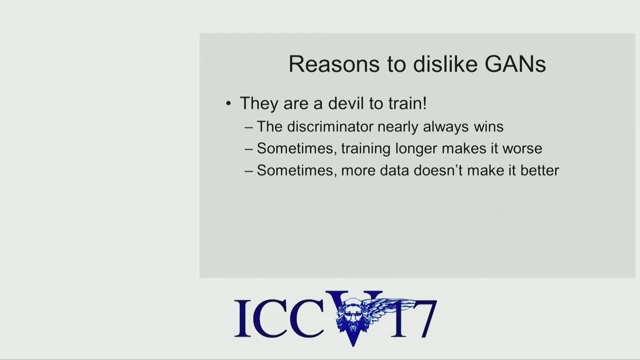 But I really hope that these things could be nailed one way or the other. So please keep working. Do they really generate a distribution? Some of you machine learning people might have a heart attack. Oh no, it's not a real distribution. 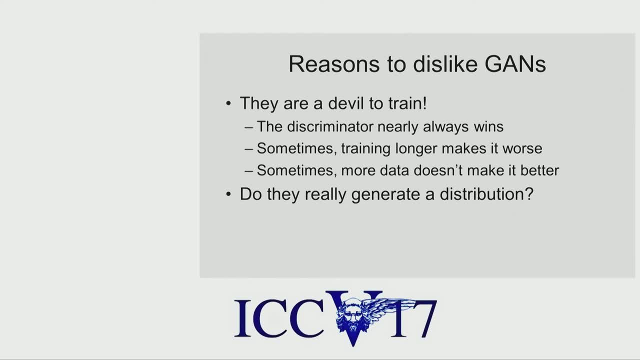 For me we don't care, We just want something to work. You know, in computer graphics you just need one good picture. You don't need the whole distribution, You just need one good one, you know. So for that GANs have been really working very well. 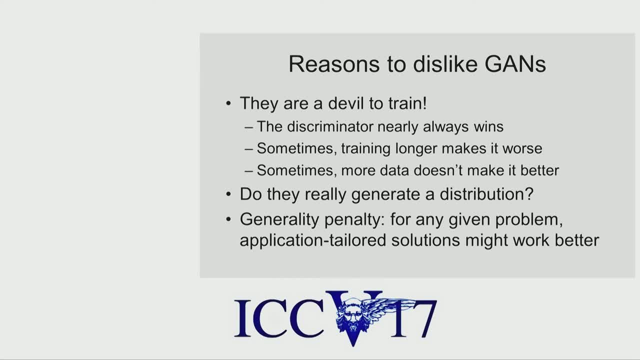 And you know there is the generality penalty For any given problem. it's often, you know, one can often find a kind of spatial tailored solution that would work better. So if you, you know, if you have like some problem that you want to solve, 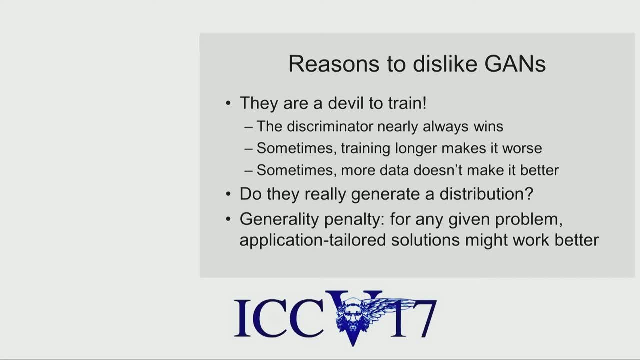 I would say, you know, try something kind of direct and straightforward first, But if you are kind of more interested in this, in this direction, I think then you should stick around. So here are my three reasons to love GANs. 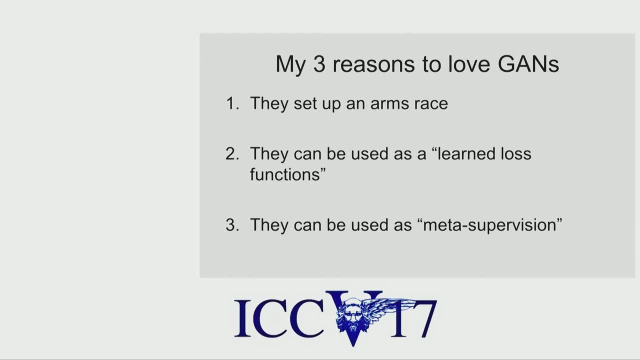 They set up an arms race. They can be thought of as learned loss functions And they could be used in meta supervision, And I'll very briefly go over this. So the first point is really very, very important. It's very philosophical. 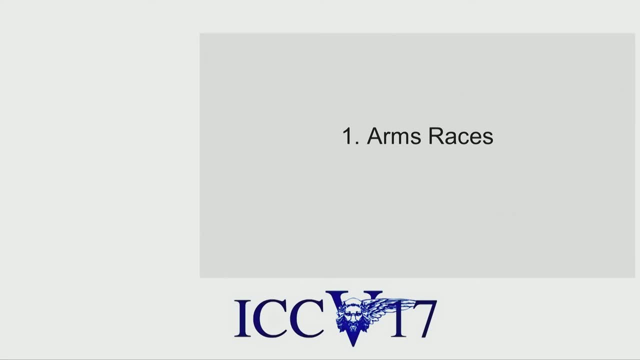 But, at least for me, that's what really got me excited about GANs: The fact that they are really, you know, an adversarial algorithm that sets up an arms race, And it seems to be working, unlike many of the others. 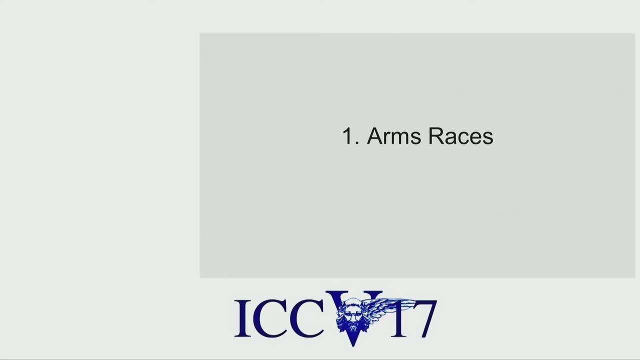 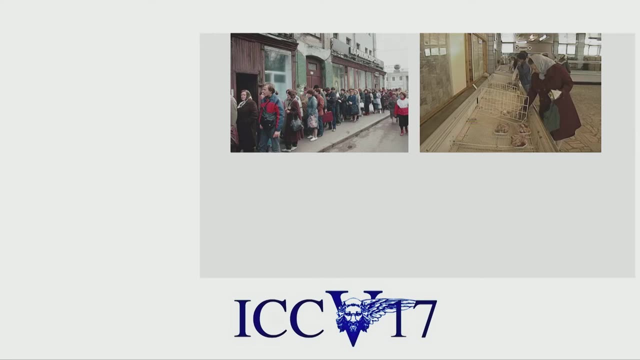 So what do I mean by arms races? This, you know, brings me back to I was. I grew up in the Soviet Union in the 80s And you know we didn't have much food. You had to go to the store and there would be either nothing or you were standing in a long line three hours to get toilet paper. 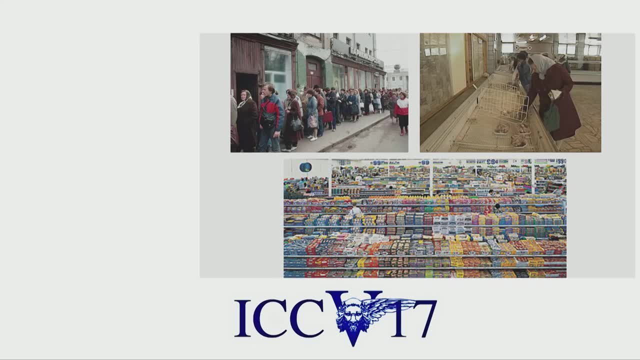 And then in the late 80s I moved to the United States And it was a shock. You go to the supermarket and there's all this stuff- you know as much toilet paper as your heart would want- And this was really hard for me to take as a Russian. 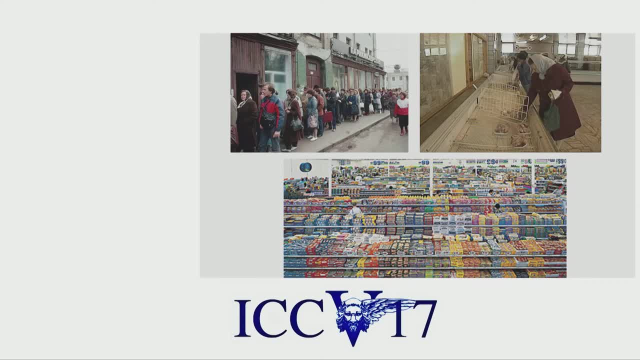 Because, like you know, we Russians we're not like super stupid, right? You know, we have great physicists, great mathematicians. you know Tchaikovsky, you know artists, writers, Tolstoy, Dostoevsky. 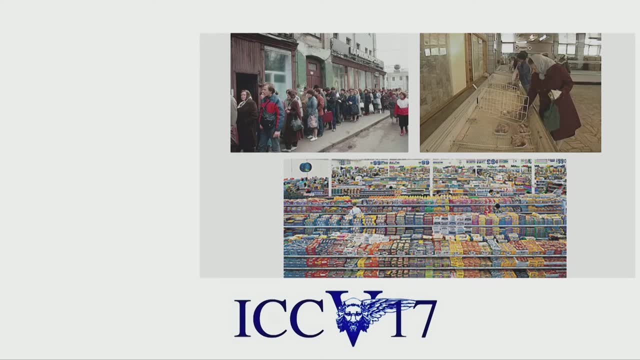 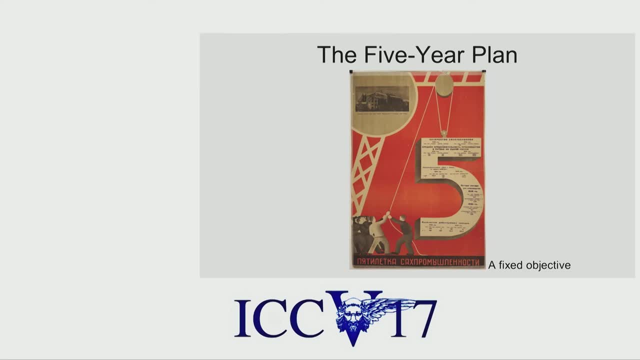 You know why couldn't we figure out the toilet paper? So you know, I read up on this And you know the one issue. that was that you know, we had the planned economy, We had this what's called the five-year plan. 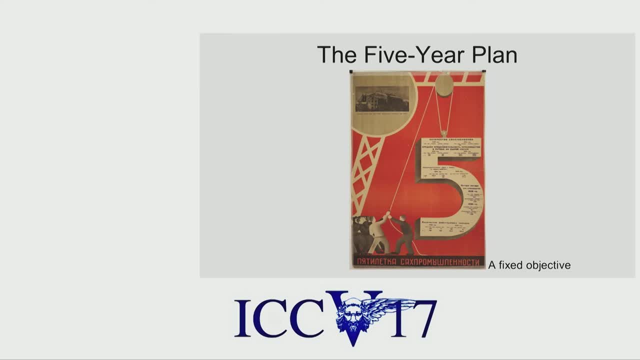 So every five years, you know the economists would get together and figure out. you know a fixed objective that the whole country would. you know how much of everything will be produced within the next five years. So it was all fixed. 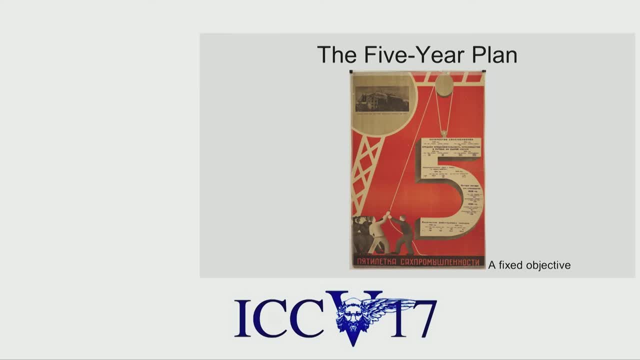 And then boom, boom, boom, you know they would do it, And that is turns out to be a problem. And to show you, here is an example of pocket calculators. So this is a famous HP-80 pocket calculator circa 1973.. 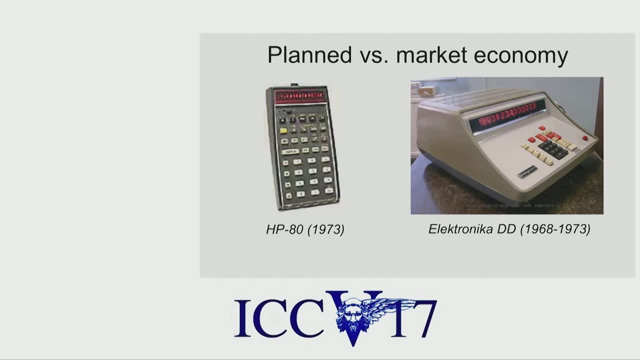 And this is the corresponding Soviet version. We say that you know, Soviet pocket calculators are the largest pocket calculators in the world. But you know why did this happen? And one reason is very likely That what happened was that in the beginning calculators didn't. you didn't really care about calculators being small. 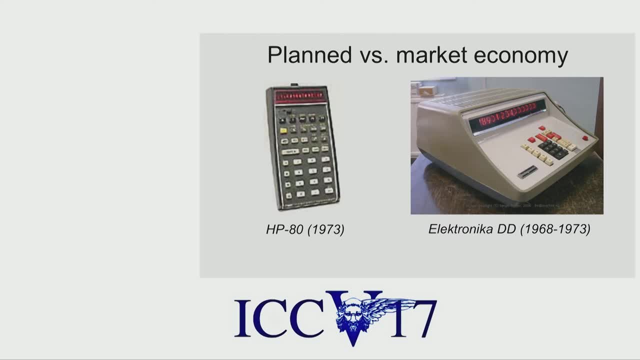 You just needed them to compute stuff. But HP was under pressure to make it cheaper, you know, And so other. so they would say, okay, how do we make it cheaper? Well, if we use less stuff, less material, it will be cheaper. 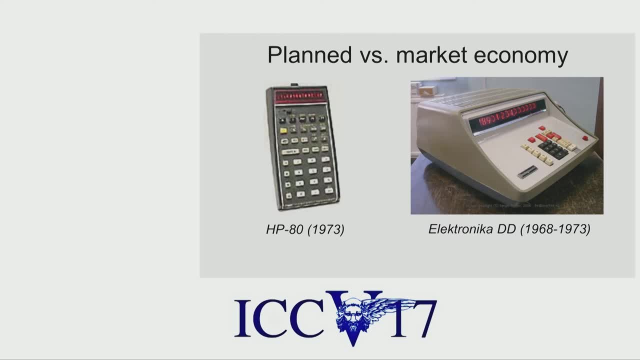 And so they made it a little bit smaller, And then other companies made it a little bit smaller, And then boom, boom, boom, boom, boom, boom and arms race developed. And then at some point they were almost small enough that people would look at it and say: oh, wait a minute. 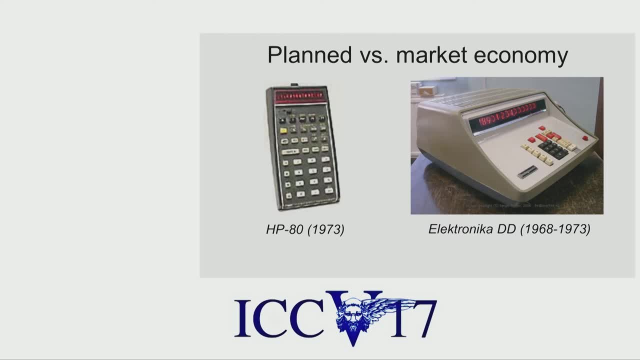 We could put it in your pocket. So basically, this arms race caused an emergent property that in the Soviet economy you never had to worry about that Because that was not the original plan five years ago. to make it small, Right. 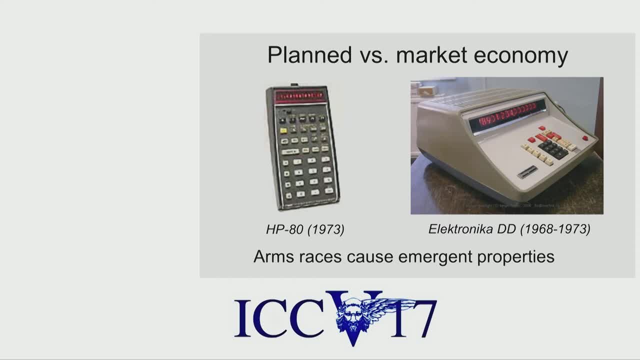 And it nothing really emerged. And so to me, as somebody who kind of suffered through the, through the planned economy, I thought that this property of GANs, as you know, as an example of an adversarial algorithm, was very exciting. 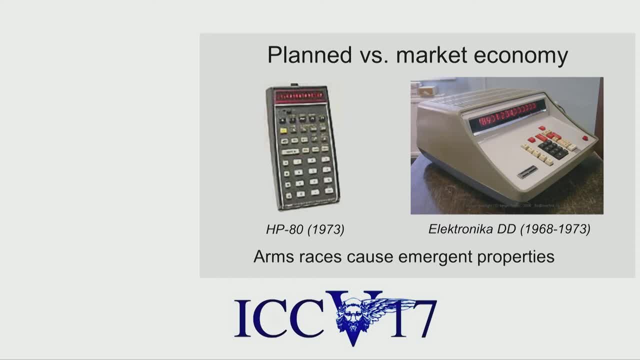 And of course there could be other adversarial algorithms out there, But I think so far the GANs are really the only thing that can really we can say is working. So I think this to me was kind of a philosophically a very exciting thing. 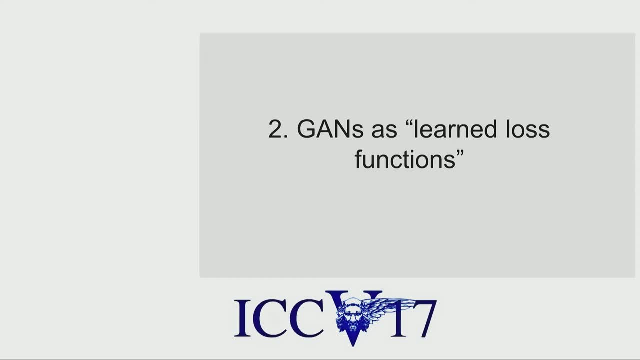 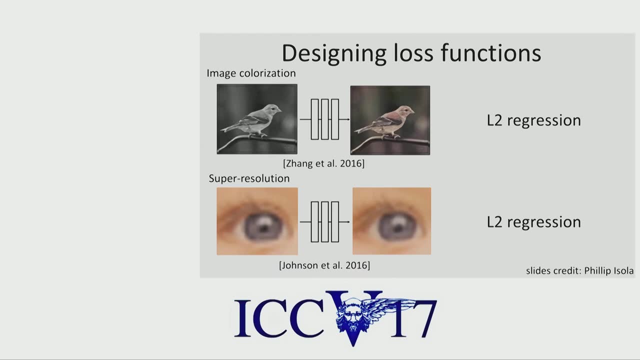 So related to this is the idea that GANs, at least conditional GANs- you can think of them as learning, Learning a loss function. So what do I mean by that? So you know if you want to do some sort of an image-to-image translation problem, for example. 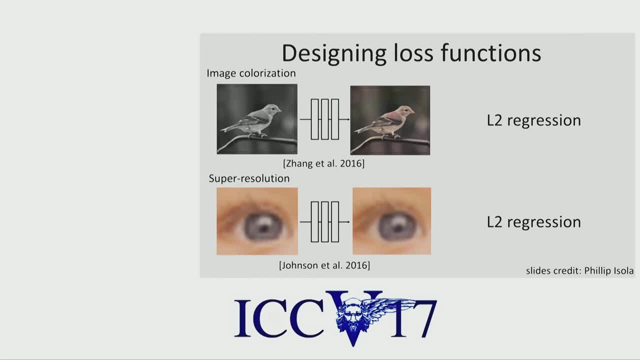 you want to go from grayscale image to color image or from low res to high res. You know you can set up a network to train it with some loss function. You know you can use L2 regression. That's what the statisticians would tell you to try first. 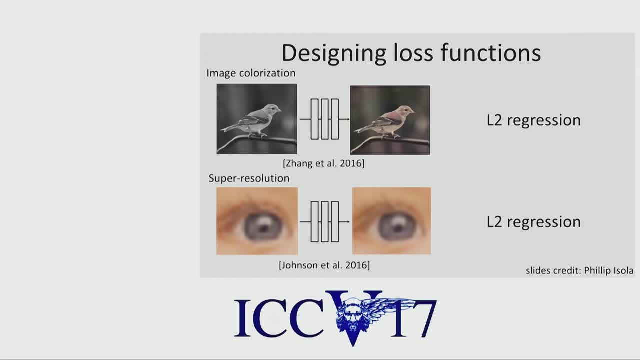 And you notice that it just doesn't work very well, Right? So something like L2 or even L1, basically it would average different modes of your solution. So you know, the bird could be red or the bird could be blue. 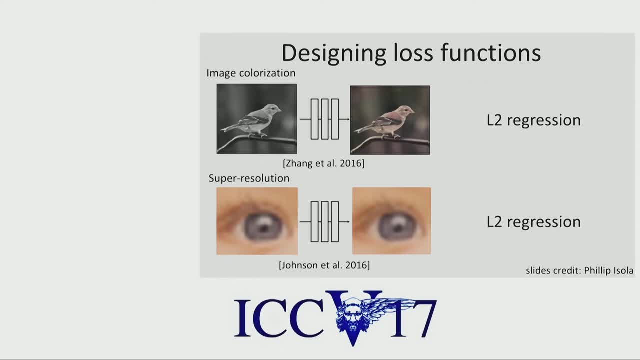 And then L2 would basically say: well, I'm going to make both of you guys happy, So it's going to be gray, just so it's. you know, equal distance from all the right solutions. But that's not what you want. 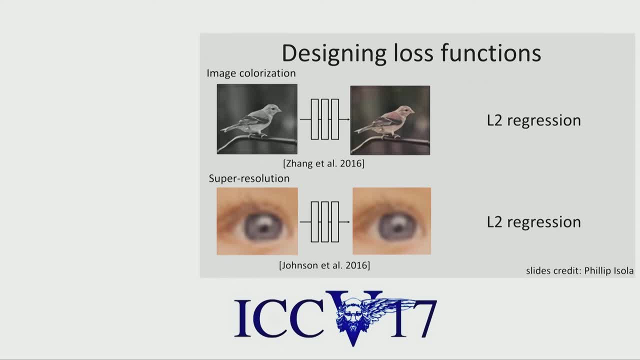 The same thing for super resolution is: just blur things together, Right, Because it's going to try to find basically something in the middle that makes all the modes happy, Even though that's Very low probability of this thing. So you know what do you do? 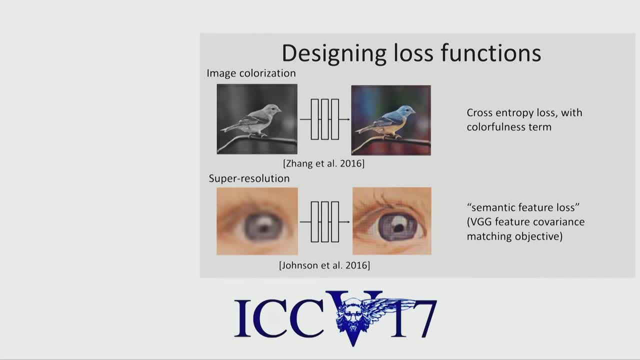 You get a very, very smart Berkeley graduate student or a very, very smart Stanford graduate student And they hack and hack and hack until they come up with some nice loss function. that works very well for this project, But then doesn't really translate to something else. 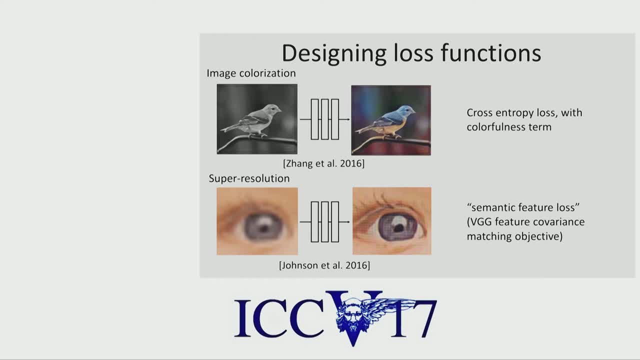 So you know we came up with this cross entropy loss with some polarization term. You know the super resolution. People use the feature loss But then you know you couldn't. They're not interchangeable, They're really tailored to the program. 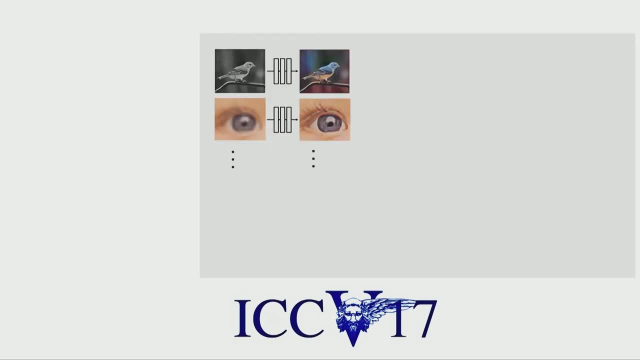 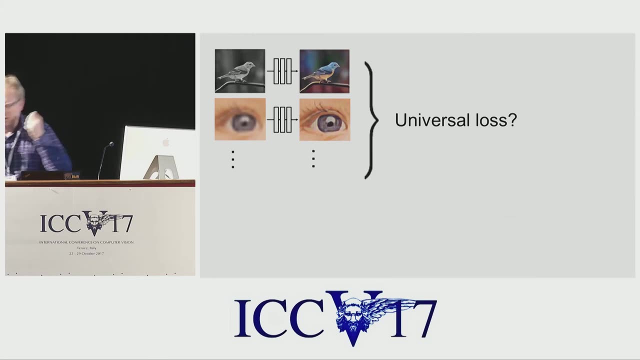 But it would be really nice to have some sort of universal loss for these kind of image-to-image translation problems. You know basically something to tell you if your image is good enough or not, And we know one such universal loss. That's called graduate student descent. 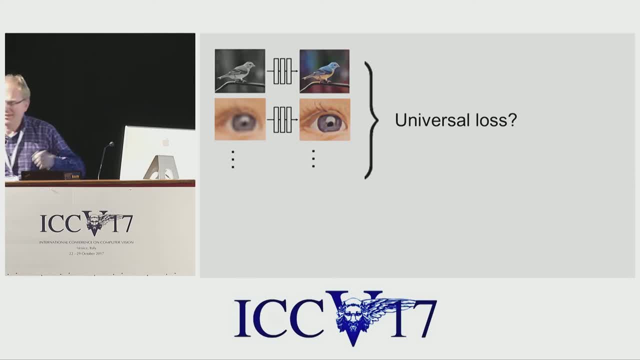 Right. You know, in computer graphics at least, you know, basically the graduate student works on this Right And basically the graduate student works and works, and works until it looks good enough to publish Right. So that's basically what we want. 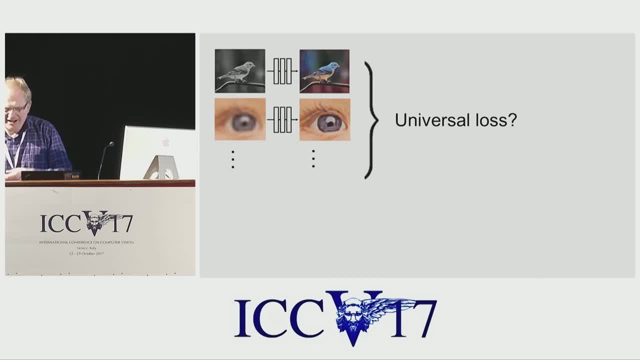 But of course it's kind of hard to you know back prop graduate students. So you know what we do for evaluation at least is we take those results and then we compare it to. you know, real photographs, Right. 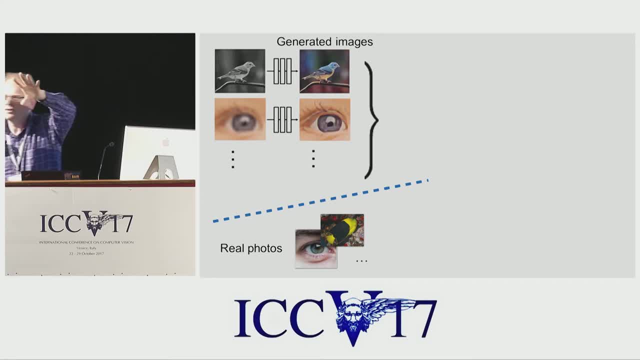 And then we send it on Turk And then we can compare: Okay, Is this colorized image? So you can be mistaken for a real color photograph, Yes or no? And that's what we report in our papers. Right, And actually, so that you can think of, the GANs is basically doing that, but instead of having it done by the Turker. 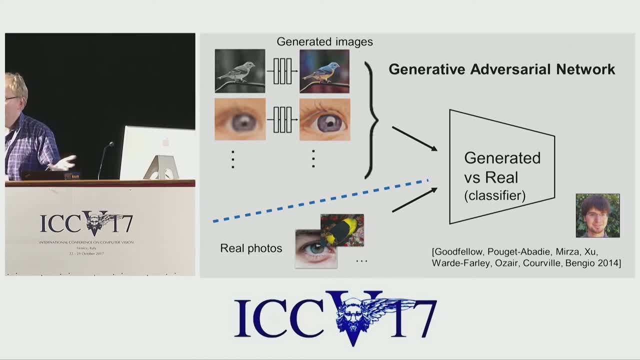 Right, You do it in the by the generator, by the discriminator, And then you can back prop for the whole thing. So in a sense, if you think about it from the point of view of a computer graphics researcher, GANs have exactly the right loss function for doing computer graphics. 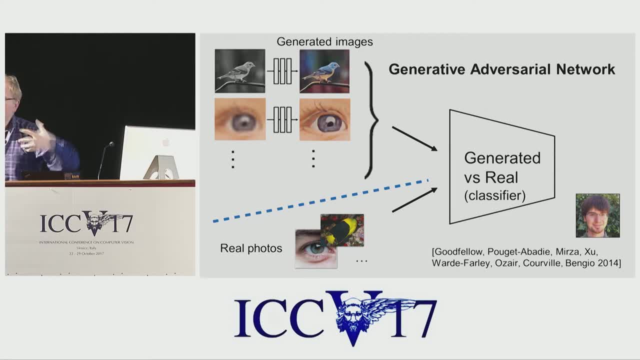 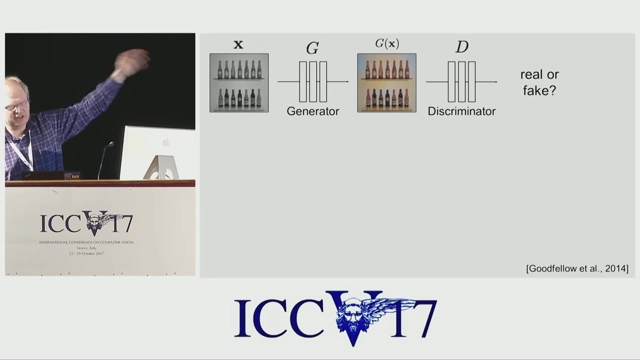 They are exactly doing what computer graphics is trying to do. Right, You want to generate samples that are indistinguishable by, you know, your movie audience from the real thing, And so that's what got us very excited. You can, you know, this is kind of the standard, you know. generator discriminator. 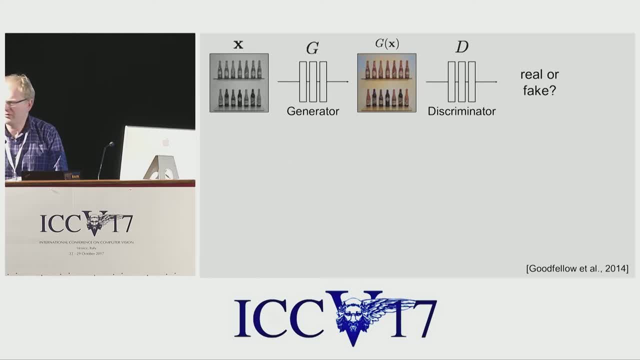 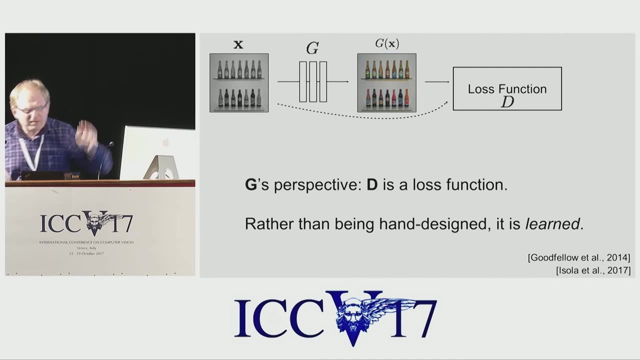 Of course we were using the conditional version of this because we want to do translation from one to the other And you know the standard, the standard story. I think one thing that is nice- and you know, Phil Phil Izola likes to point this out- is that from the point of view of the generator you can think of the whole discriminator. 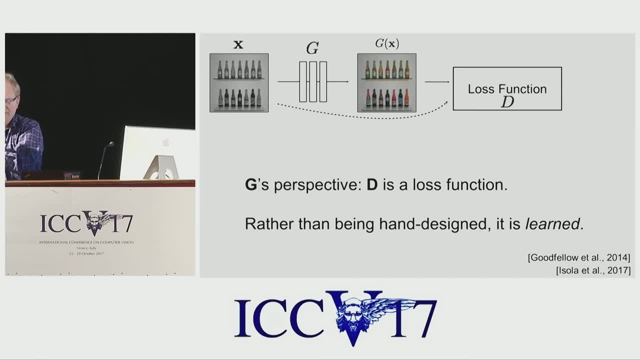 That whole thing is basically just like a loss function, Right, It's not quite a loss function, but you can think of it as a loss function, except that instead of like L1 or L2, it's a learned loss function, Right? So, basically, what this thing is doing for you, it's giving you a learned function for your particular task, tailor-made. 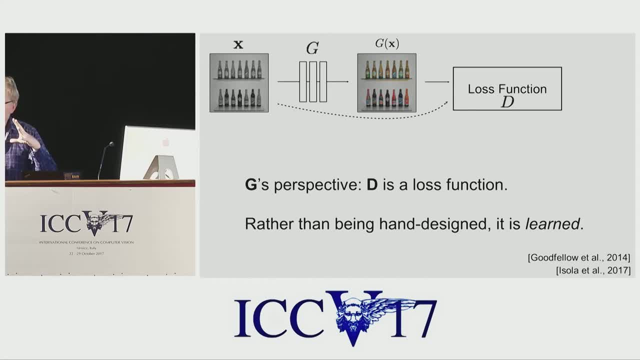 And the nice thing is that this loss function is actually, you know it has some emergent properties, You know Whereas you know L1 or L2, it really looked at every pixel independently. It doesn't really look at things, the interaction between pixels. 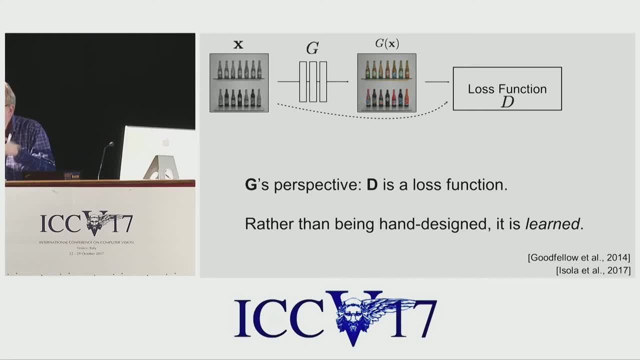 This thing. if it needs to, it will encode these. you know it could be a structured loss. if it needs to, It can do very sophisticated things kind of on its own, And it's kind of a very neat trick that you can basically, you know, just for a given input-output domains, you get your own tailor-made loss function, basically for free. 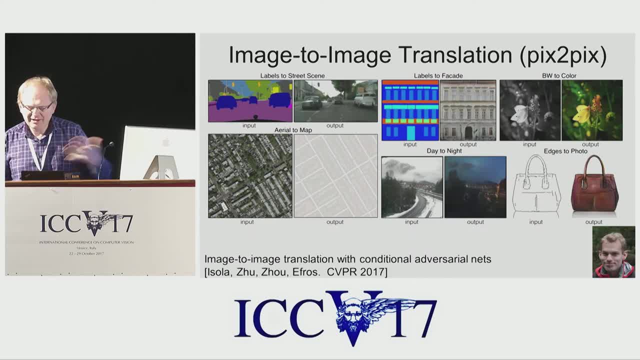 And so that's one way to think about, kind of, why we were getting this kind of cool results on stuff that Junyan just talked about earlier Without really changing anything of the algorithm. It's exactly the same algorithm, Even exactly the same parameters. 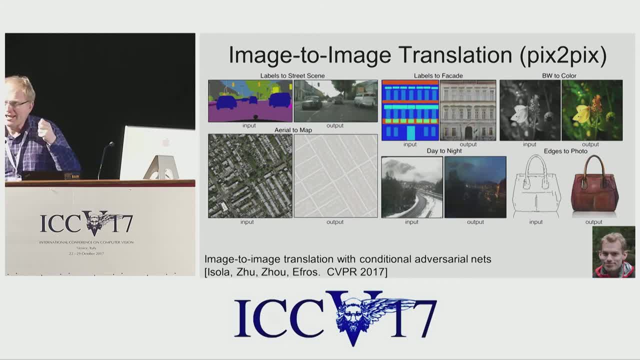 So the magic is in this, in GANs, basically getting you figuring out for every domain pair, figuring out the loss. that would, you know, do something reasonable. And again, you know, for any one of these examples you could sit down and come up with something tailor-made that could work as well or even better. 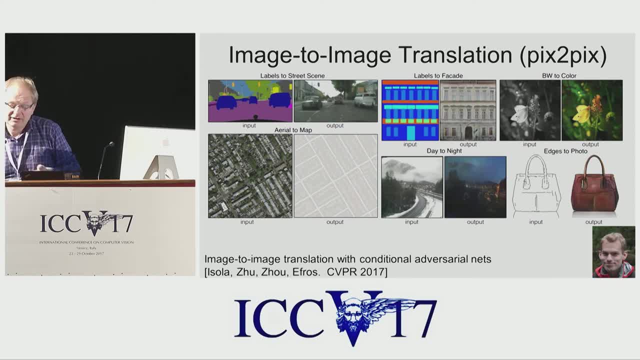 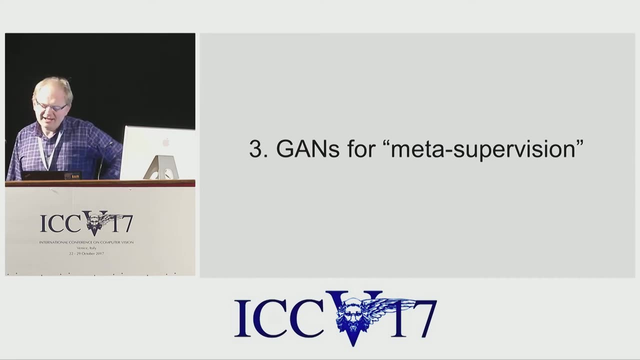 For example, for colorization. you know our other results are better, But really nothing, really Nothing really seems to work as good on just all of the things altogether, And this is, I think, very exciting. So the third point is GANs for meta-supervision. 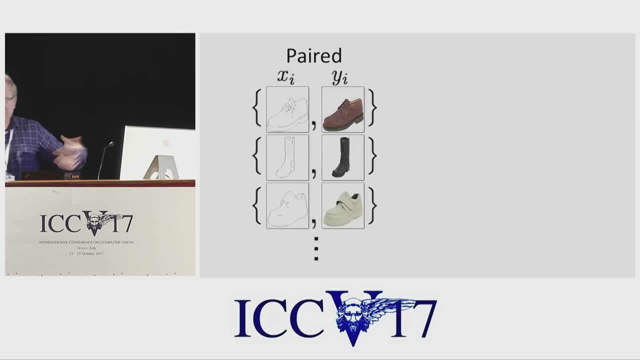 So what do I even mean by meta-supervision? So kind of motivation here is that for Pix2Pix you have to have paired data. You know, you train your. you have to pair your sketches to your shoes, for example. 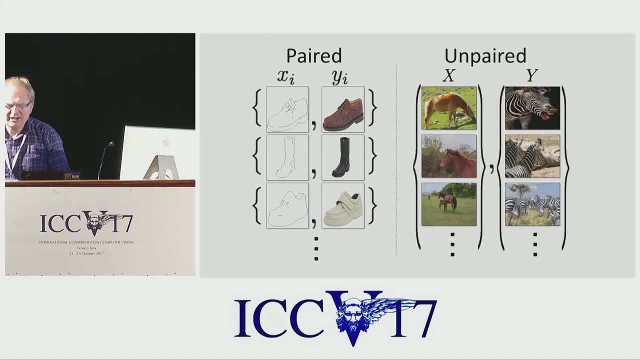 And then you can generate things right. But what if you don't have the paired data? So, for example, if you have you know a set of, say, horses and a set of zebras, right. Or a set of you know photographs and a set of Cezanne paintings, right. 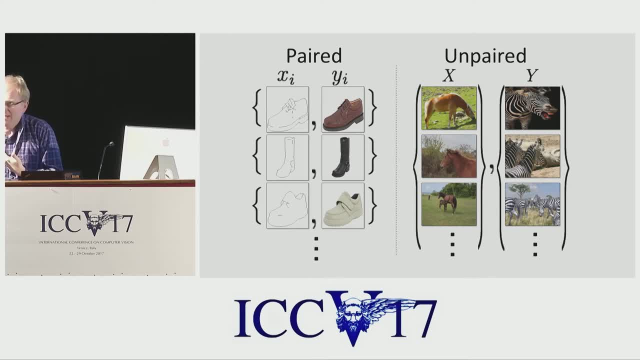 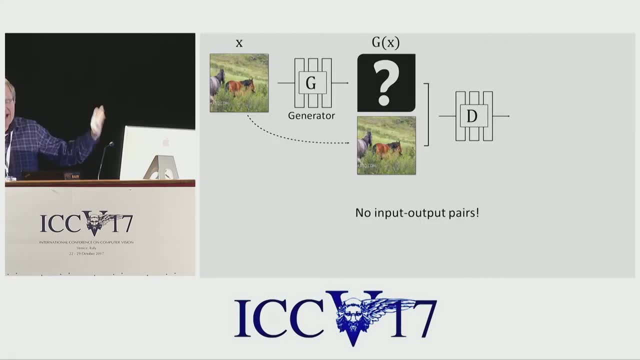 There is no. it's not even clear how do you make the correspondence. It doesn't even make much sense. So if you do that then the whole kind of standard GAN story doesn't quite work out, Because you know conditional GAN, you really need to have the kind of the input image. 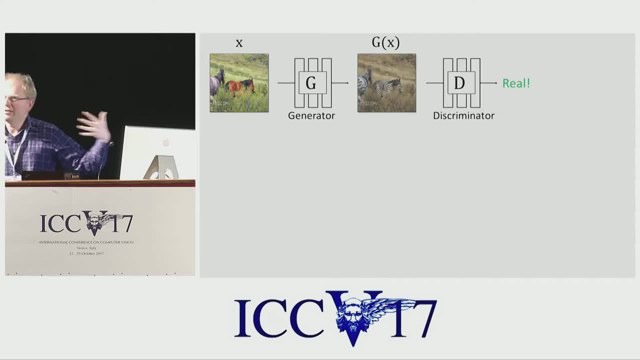 But in if you don't have. if you don't have a correspondence, then okay, So you can put a discriminator and say, okay, you know, this is a horse, this is a zebra. You know, this zebra looks good to me. 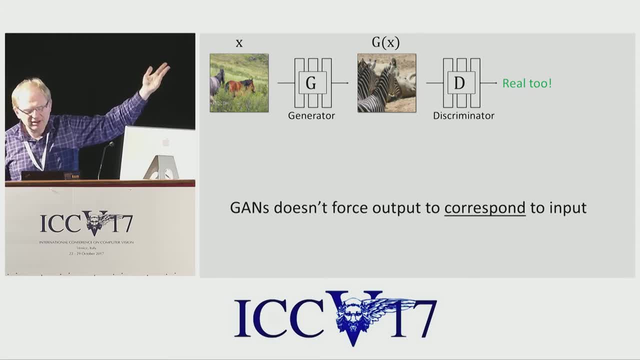 But you know, so does this zebra right? This is also real, And the discriminator would be just perfectly happy with this zebra. that has nothing to do with the input right, And so The problem here is that, basically, we somehow need to get this correspondence between the different domains. 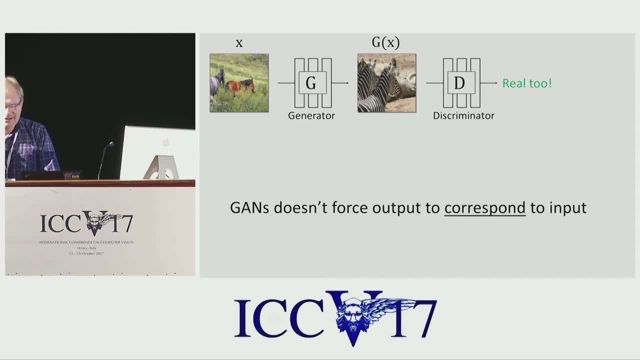 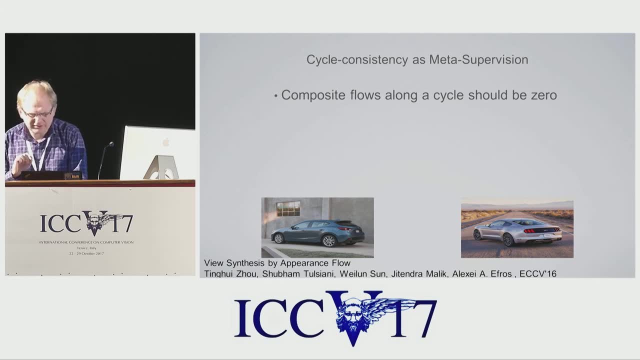 And this is something that we have actually worked on before. Now, this has nothing to do with GANs, but it turns out to be relevant Basically for correspondence. we can think of this idea of cycle consistency, Where we can composite. 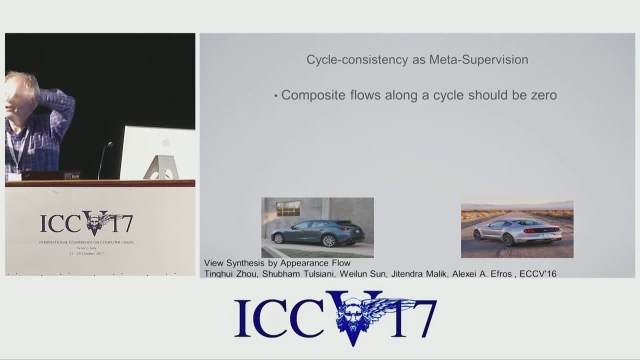 Composite Optical flows between sets of images to see if they are consistent with each other right? So in this particular paper we're looking for, you know, consistent between different instances of cars. So basically you can think of it as looking at a consistency of flows going one way and then going another way. 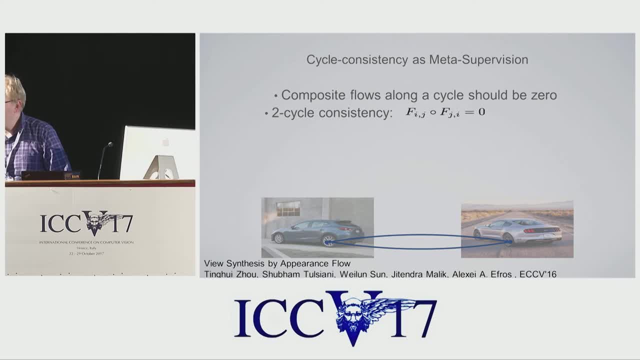 And if you go there and you come back you get to the same place, then you're consistent, And if you don't, you're not consistent. And this has been used in computer vision for a long long time. You know tracking. 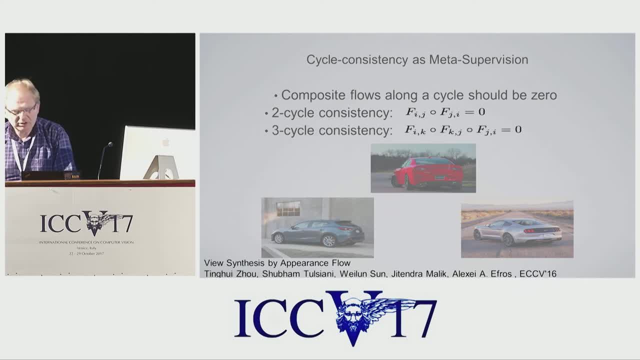 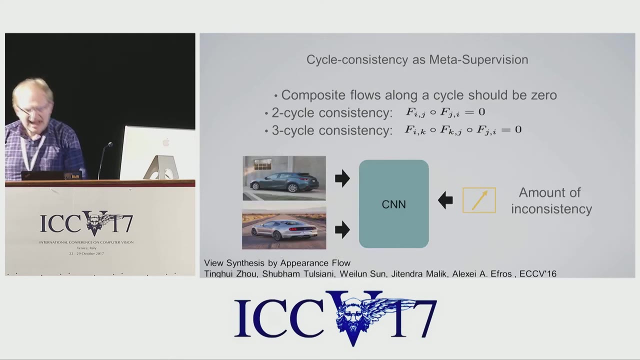 You forward track and then you backward track, for example, But you can actually use it for multiple examples. Still the same thing. Consistent, Not consistent. And. But the cool thing is that the error between where you start and where you end up can then be used as a signal to train your CNN. 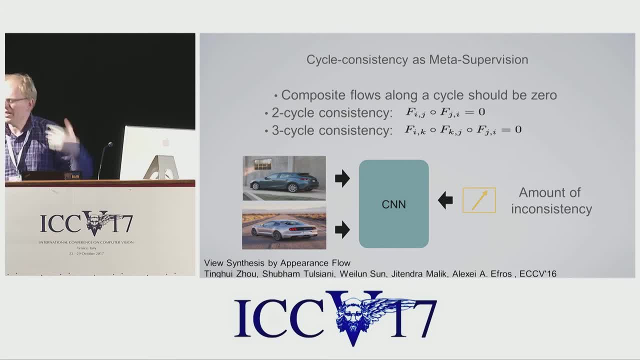 Okay, So this is- And that's why we call it- meta-supervision, Because what you're doing, You're supervising This- is not, you know how, what the data should be, But how the data should behave. 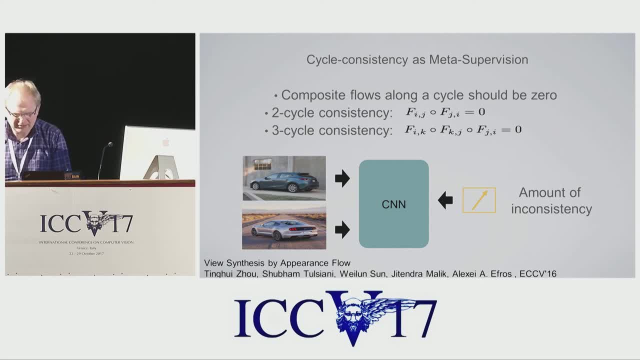 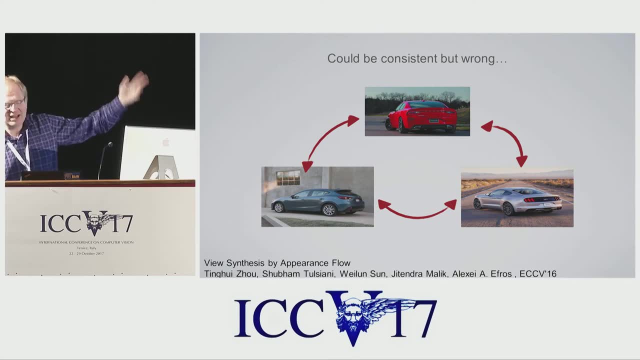 The properties of the data. In this case, cycle consistency is a property of the data that you wanted to have. But the problem with just using cycle consistency by itself is, you know, it could be consistent, but wrong It basically can be, you know. 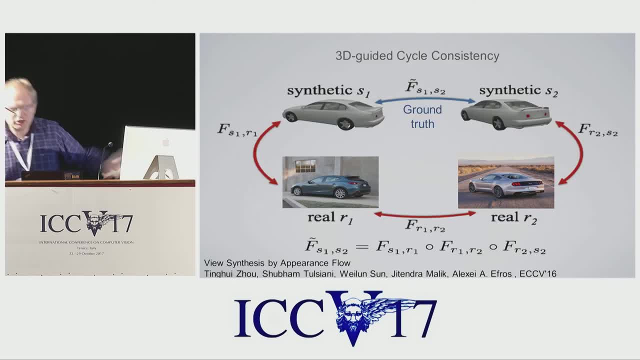 The flows could be all zeros and it would be perfectly happy, Right Um is, we actually went to a you know 3d model and then we made some real ground truth correspondences as an anchor to keep it in place, and then we we optimized for the other uh correspondences. 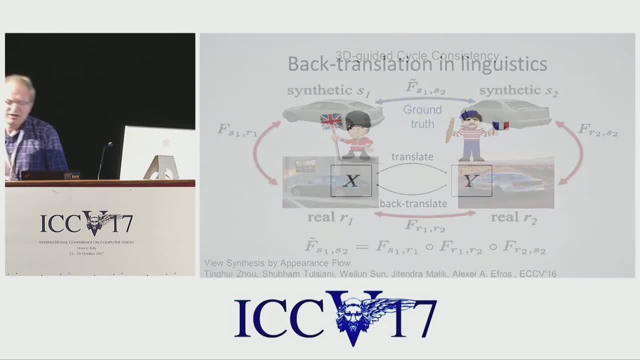 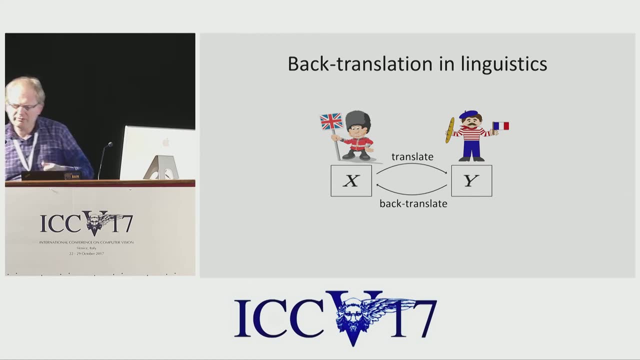 but sometimes you don't have that anger. what do you do? so? another place where this cycle consistency is being used a lot is in linguistics, in this idea of back translation. uh, it's often used when you have to say something very, very important, like pharmaceutical, you know, documents. 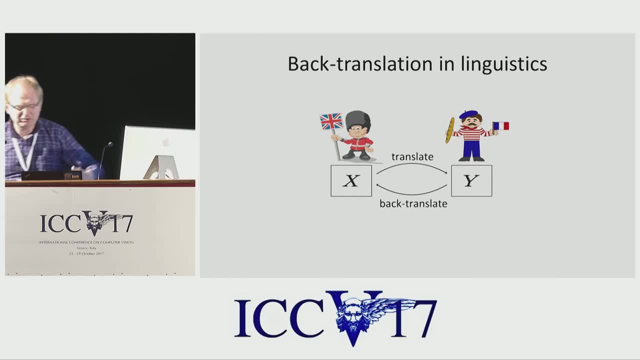 so you have you. so you know your pharmaceutical document in english and you want to translate it into french, um and uh, but you need to make sure that it's exactly the same thing. so you, what you do is you hire another uh translator and that person translates it back into english and then 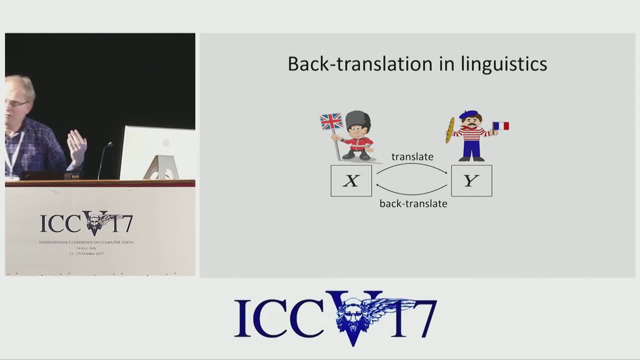 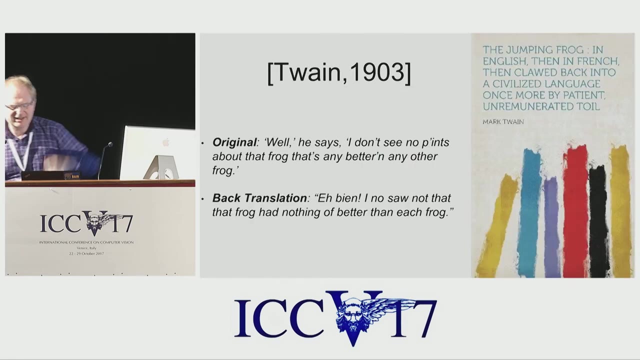 you compare um the results of of the translation, and that that's why you make sure that it's correct translation, or if it's not, then you can update it. you know and and and you know, basically figure out until it converges right. so that's the idea in linguistics. uh, famously it the the work. 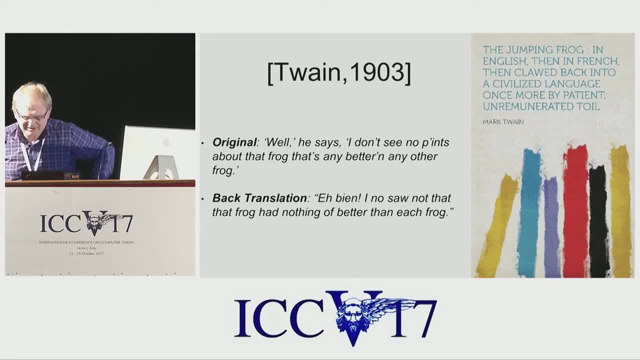 started with mark twain, 1903. this is, this is a paper he wrote, the jumping frog in english, then in french, then clawed back into the civilized language once more by patient, unrenumerated toil. um, it's a, it's a quite an entertaining thing on the failures of, of translation. uh, but the point. 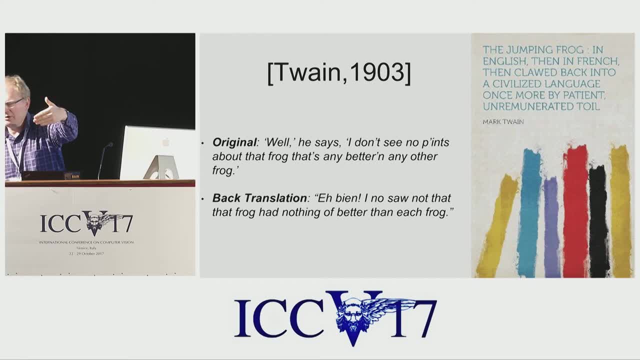 here is that, even though you know you, you do this kind of cycle in from, from one language to another. how do you know that the other language is actually french? well, in, in terms, in, in. in the case of translation, you know, you could always just evaluate whether the resulting french 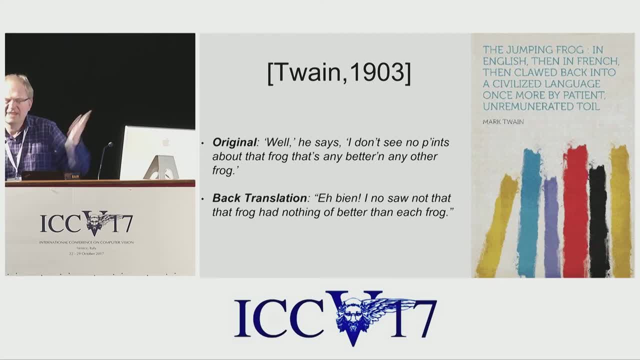 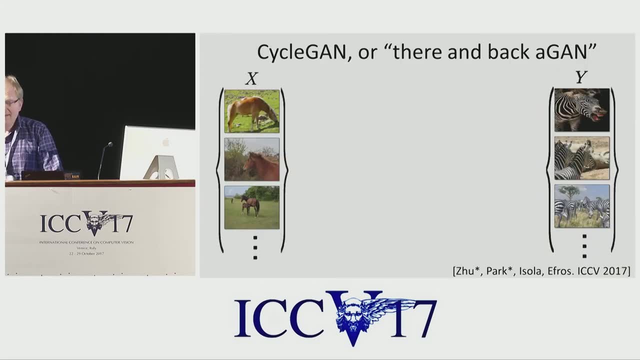 language is actually correct, french, right? uh? and that's kind of a kind of standard, given thing that that is supposed to be french, but in our case this might not be quite the case, right? so this is where we can set up a cycle. we can say: okay, well, if we want to. 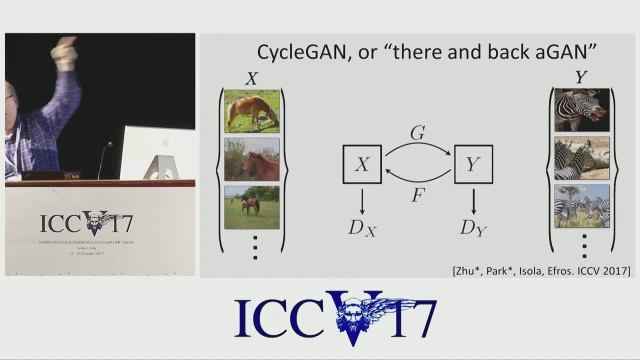 translate in from from horses to zebras. we should go back to and translate from zebras back to horses and make sure that we get something that looks like a horse right, but we also need to make sure that when we go there to the zebra land, it's actually is a zebra and not some random thing. 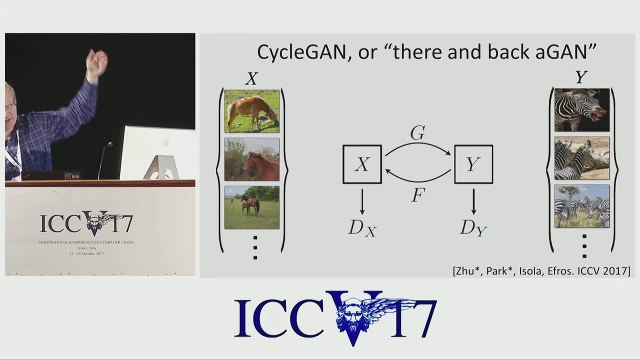 right, and we would. and you know, we want to make sure that the, the g and the f are actually not empty transformations, and so this is where we can use the adversarial loss to force this uh in in our translation, to force the other domain to be actually the correct domain. okay, and so in this sense, the, the adversarial loss. 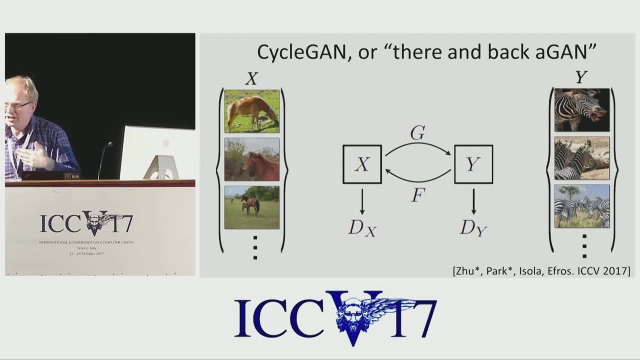 from again can act as another type of a meta supervision. it doesn't tell you what you should be, it just tells you in what domain you should be in. you know in in previous case it was you should be in the domain of natural images. here it's in the domain of, you know- natural zebras, okay. 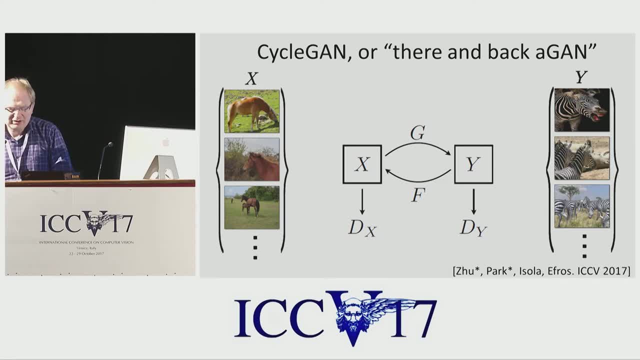 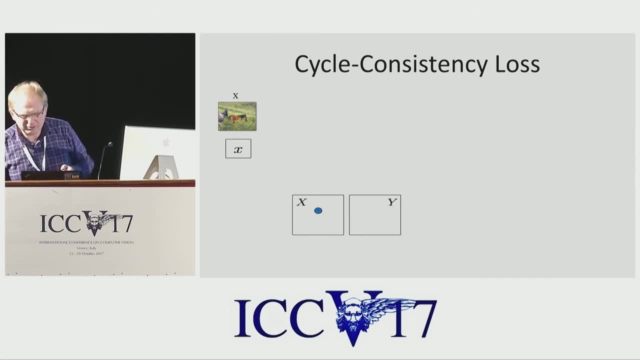 but you know, once you're do, once you've done that, it's actually pretty simple. so our whole thing is is as follows: you know, we start with our input from, you know, from a horse. then we translate it to the domain of a zebra- and this is our adversarial loss here- and then we train. 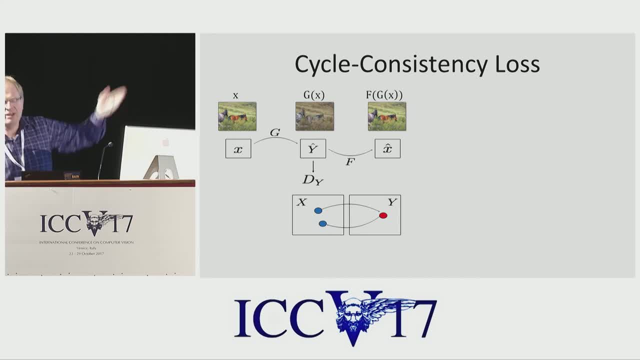 another translator to translate it back into the, into the horse, and then the cycle. consistency loss is basically just the LL one distance between where you start and where you go, and that's what you're optimizing if you, if you look at the squint a little bit and look at this from afar, this is 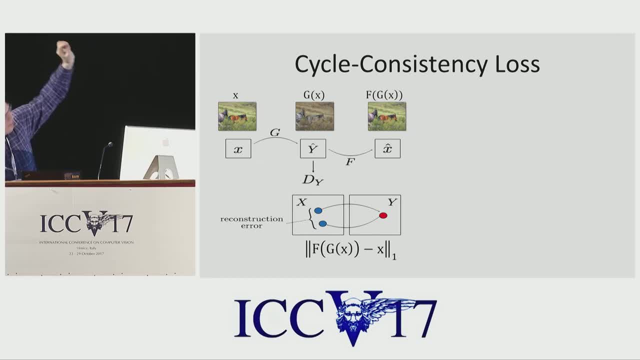 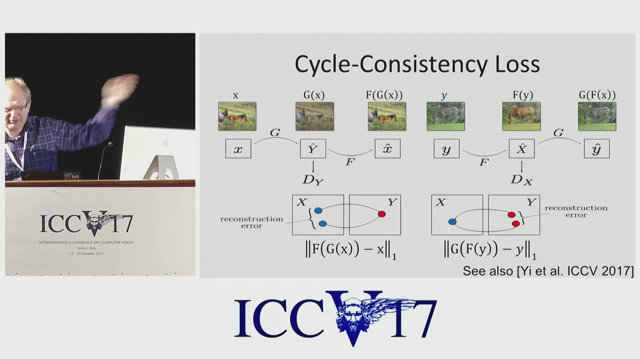 basically an out encoder, but with with a deep supervision in the middle, and the supervision is from the other domain. but other than that, it's basically kind of a standard thing that we know and love, and we do it from the other direction as well. so that it's it. it's symmetric, okay, and so we have this pay. this is, this is work we have in. 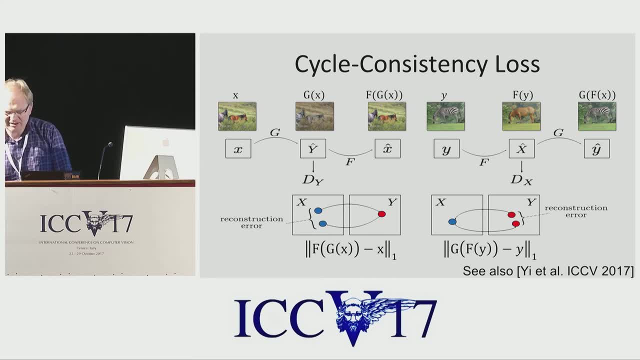 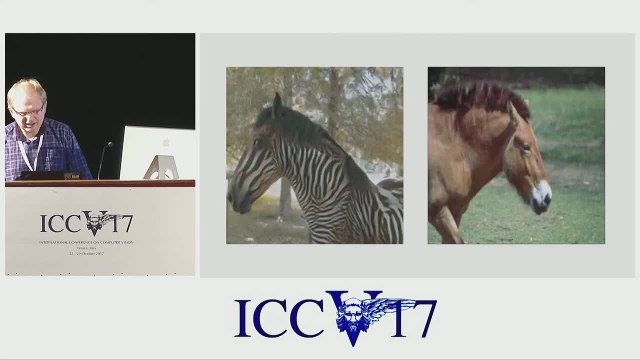 iccv and actually there is another paper that basically came up with this, the same story also here in iccv. so you know, we can convert horses into zebras, we can convert zebras into horses. it's the same algorithm, right, and notice that actually you know it makes. 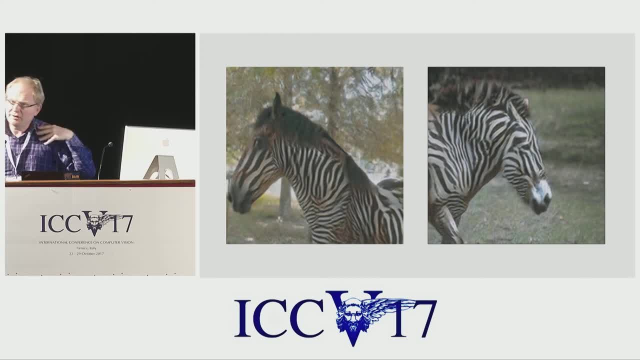 it, it, it's. it's actually solving an, you know, unsupervised correspondence problem, because it doesn't really nobody told it what the zebra is right. so it basically solves this correspondence and it sometimes it, you know it- it can also, you know, change the savannah a little bit make. 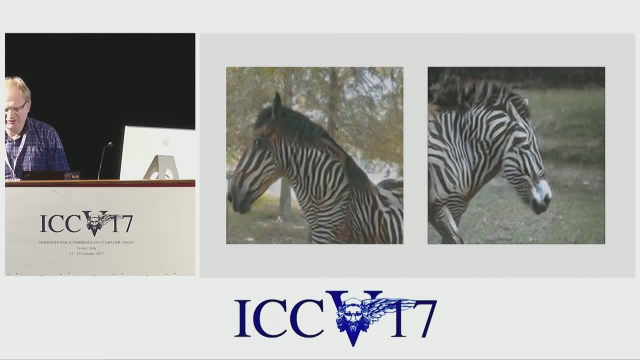 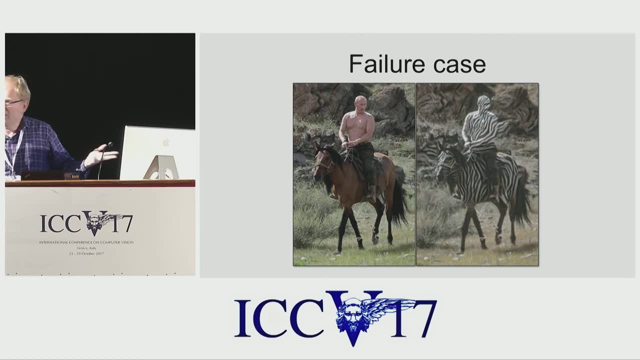 maybe make the, the greenery more yellow because of the samana, and this is also why you know some of the, some of the failure cases are kind of entertaining, right. the, the horses and zebras never saw, never, never saw a human and the zebras never saw a human and the zebras never saw a human. and 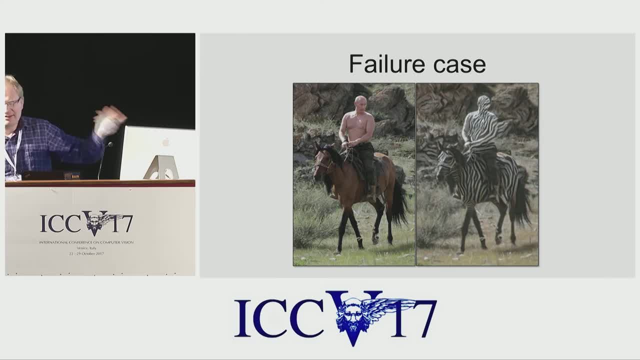 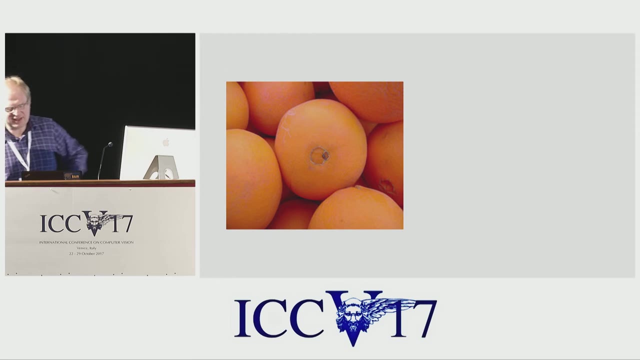 and so that is the case where the the, you know the correspondence algorithm- didn't really know what to do, so it assumed that putin here was part of a horse, which is not unreasonable given that it's a completely unsupervised problem. um, so then we can do other things like turn oranges. 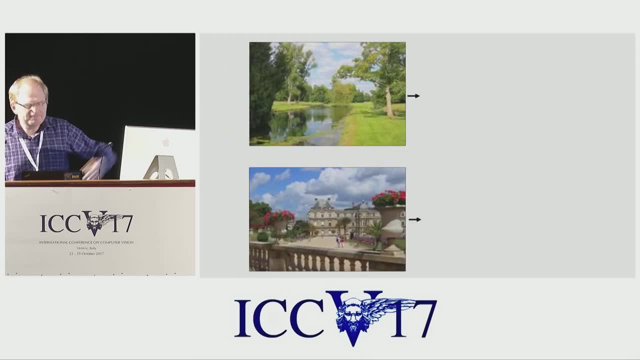 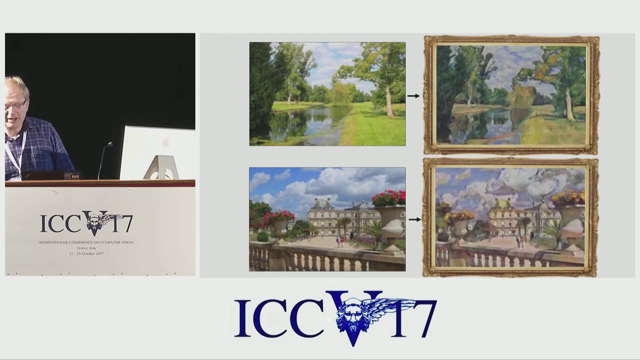 into apples and apples into oranges. uh, my particular favorite is: i have all these beautiful pictures of, of, uh, of france and i thought, oh, i can, i can try to make them look more like, you know, a cezanne painting, and indeed it actually, you know, works pretty well. 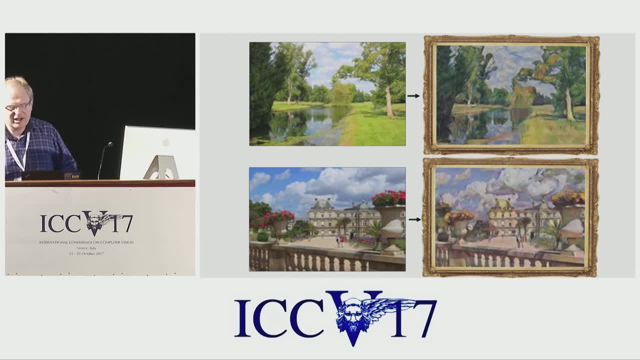 again exactly the same algorithm. there is no changes in parameters, um, and one thing that's interesting is that when we tried this on just random images from flickr or or image net, the results didn't work very well. uh, but here you know, using my pictures that i also took in france, you 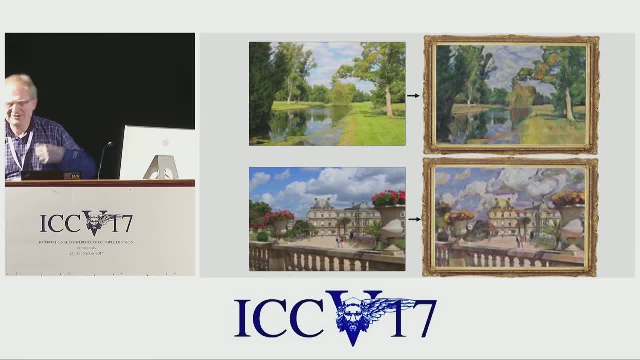 know there's maybe something about the domains being not too different, so you know it has to be- at least you know, the same country, or something like that. but i think it's, it's, it's, it's, it's, it's something like this: the results were much, much better. um, now, you have seen this kind of results. 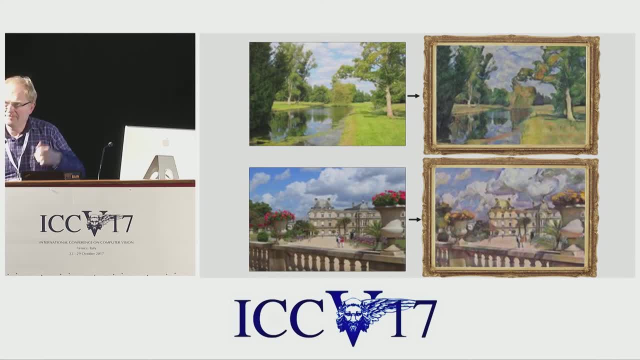 before all this, uh, you know, domain, a style transfer, kind of things, neural style transfer- i would claim that our results are are better. look, look at this. check out those uh clouds from, uh, the, the cezanne clouds there. i think that they're, they're better than what all of the, all of these? 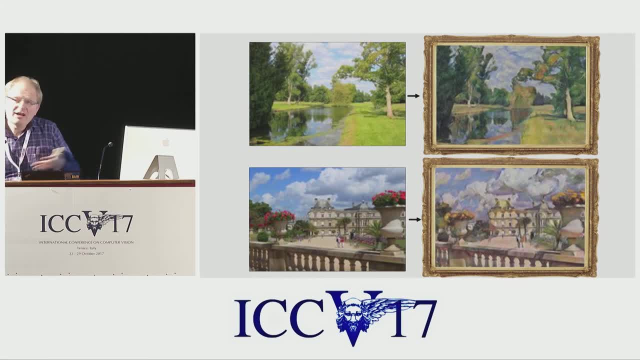 domain. uh, uh, style transfer algorithms can do in, because here we are actually looking at the whole of cezanne's paintings, not just a particular, you know, one painting, so it's able to actually, you know, gather more uh statistics about, about this issue. uh, what you probably haven't seen before is 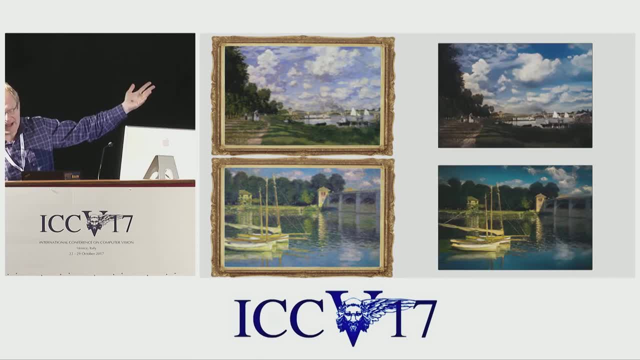 the fact that we can also go the other way around, go from a painting to something like a photograph. and here i think it's really the, the, the all, the uh. all the credit goes to gans that you know they're, i think, on the casp of getting a. 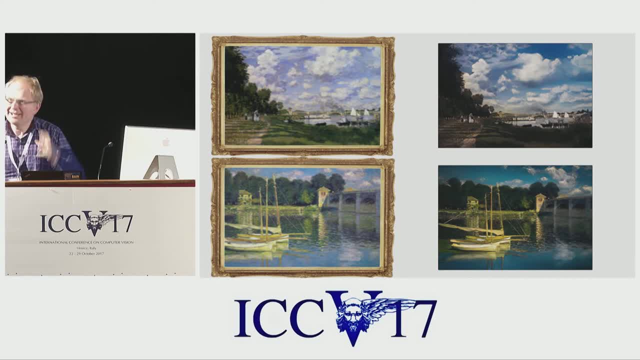 us something getting us a loss function that really can get us to almost realistic images. i mean, these are not quite realistic and you know the the input images are monet and not cezanne. it would be nice if it was cezanne both ways, but cezanne doesn't quite work as well. monet is closer. 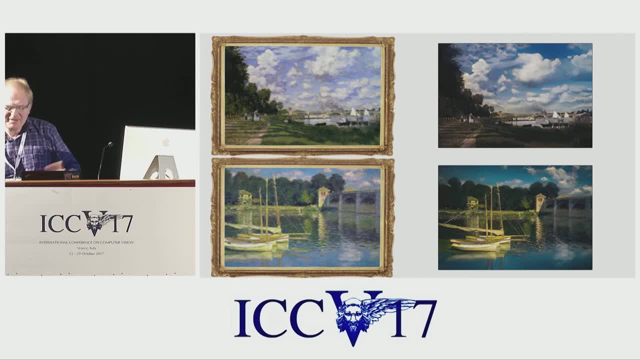 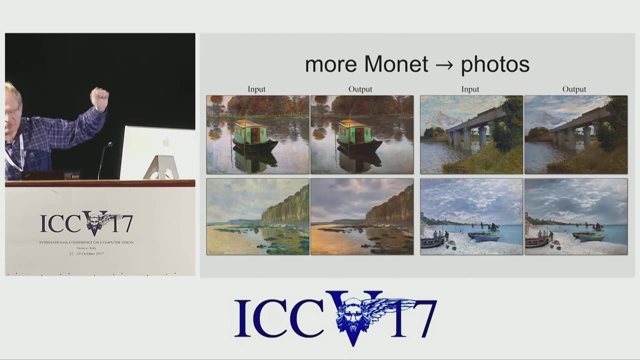 to to real realism, so it works better. but i think that's really really exciting direction and i'm sure that within a year we'll we'll have, we'll have gans producing, producing really real photorealistic images. um, here are some more examples from monet. uh, you know, there's definitely some places where 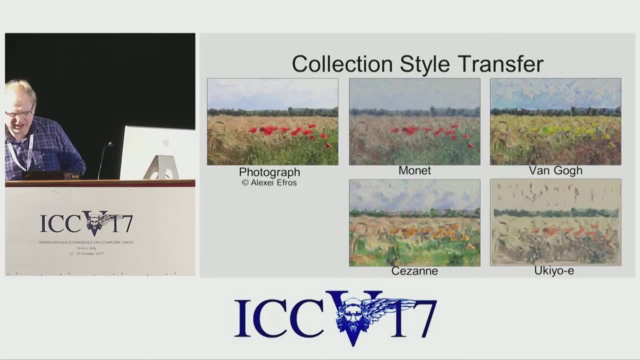 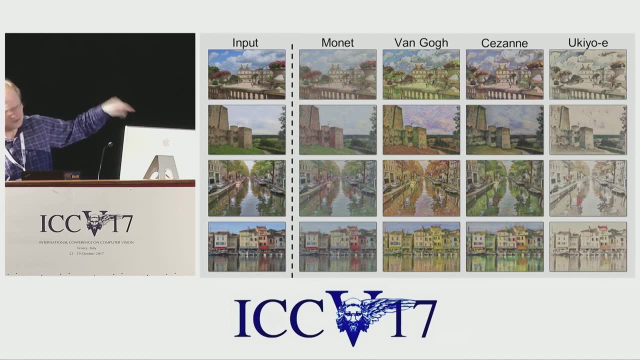 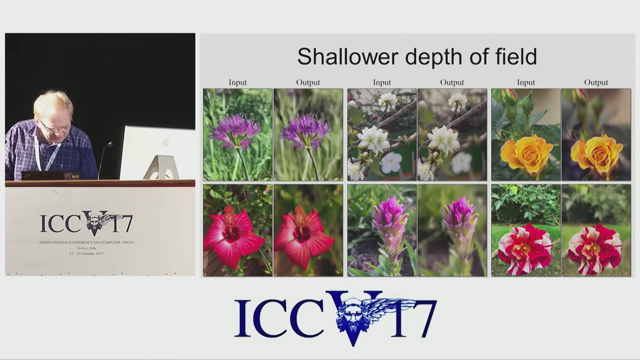 you can tell that they're not quite there, but but i think it's, it's on the right track. uh, here's some more examples of style transfer, different and this i just like to show my travel photos, for this is from eccv last year. um, so ah, i have three minutes, so i wanted to uh call my student, uh taesang here. 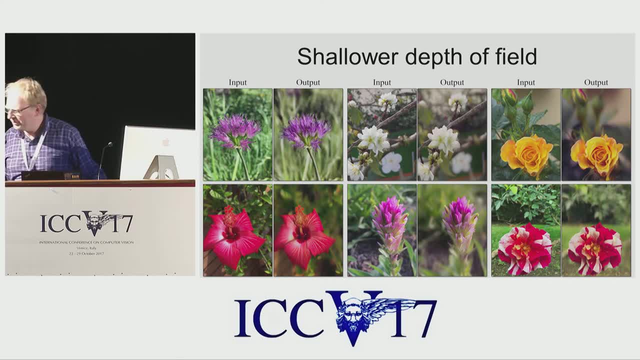 to talk about this. so today we have 26 students, uh um. the students have uh had several times uh um events, uh kind of awesome events, and and and and uh. you know that they're able to interact with each other uh develop new and new results. they're so off the heart of the press. 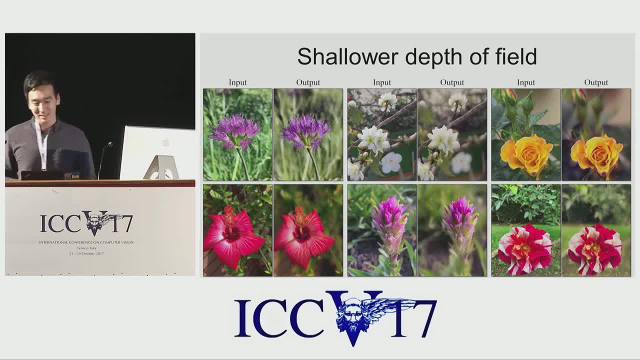 that i wanted him to to present it, uh, and then we'll be still three minutes, okay, all right, all right, yeah, so it's basically the same same method, cyclic and trained on different application. you know, different data sets. so what i did is i trained cycle again on the images taken by iphone and also the images taken with dsrls which support, which are supposed to have shallower. 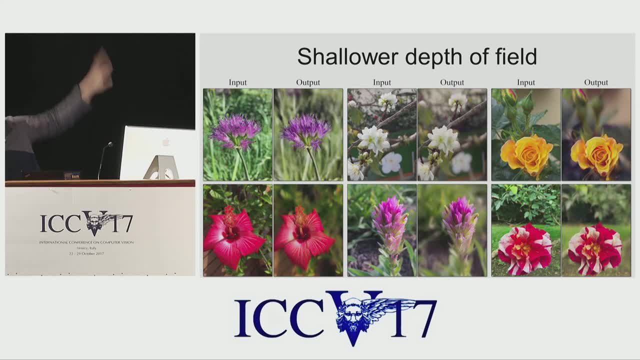 deltab field so you can see that the background of the output images are blurred. you know this is the effect that's simulated using dual camera in the more recent versions of iphone plus, which are quite expensive devices. you know what you can do: instead of buying these devices, you buy a cheaper smartphone. 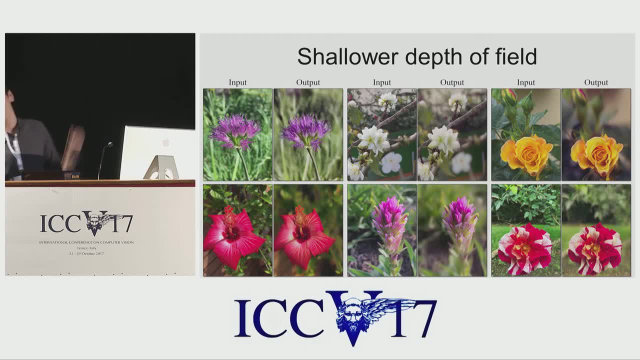 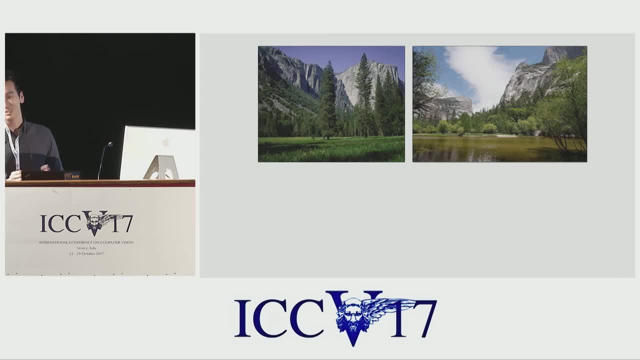 and then just build an app using cyclogan that does this for you, then you can save money or even make money out of it. i just trained it on summer and winter yosemite data set. so here we have summer photos of yosemite. we can transform it to winter photos of yosemite or we can also do it in the. 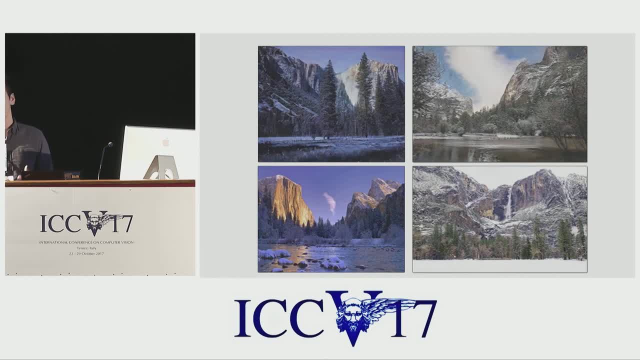 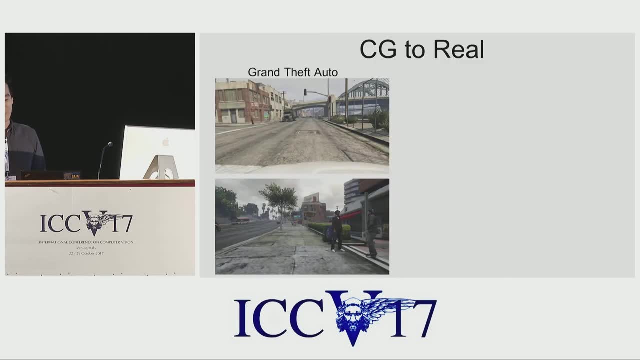 reverse direction. cyclogan is training two generators in two different directions. so, given real photos of yosemite, we can change it to summer photos. we also ran it on cg2 real. so, given screenshots of gt, a grand theft auto which has really fantastic rendering of uh driving, it's basically a cg. 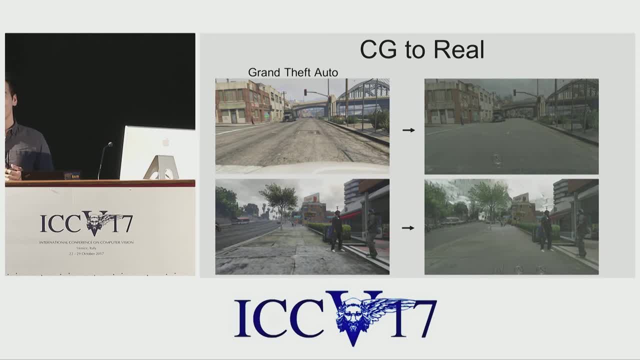 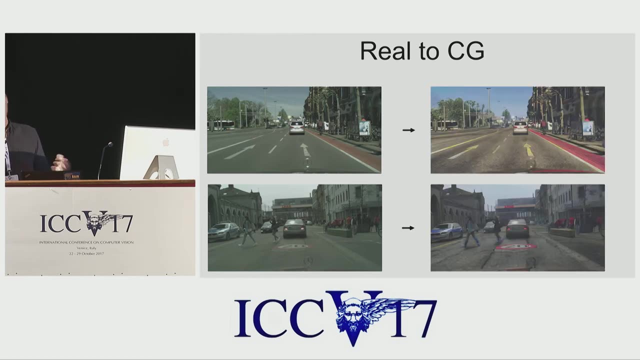 driving data set and then we can make it more realistic using uh cyclogan, trained on gta screenshots and also the real images of driving. it can also do it the other way. so, given real images of driving, we can make it more computer graphicsy. we actually created a video out of this. 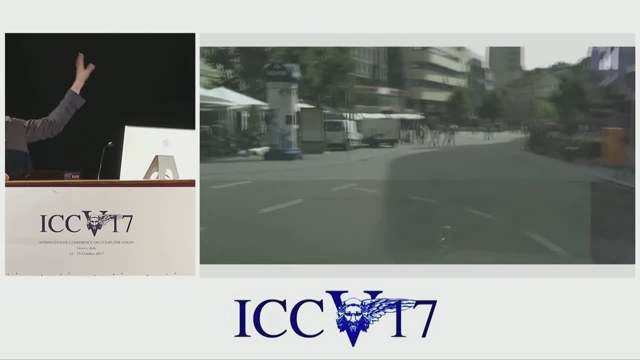 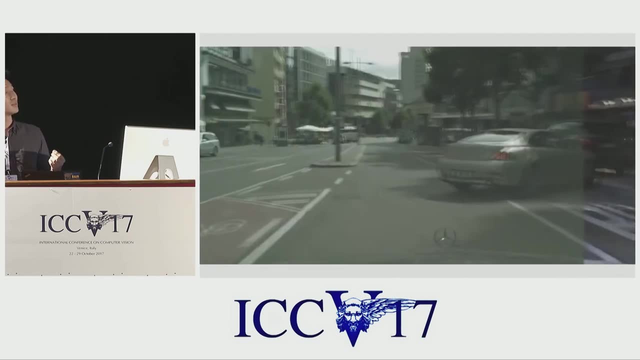 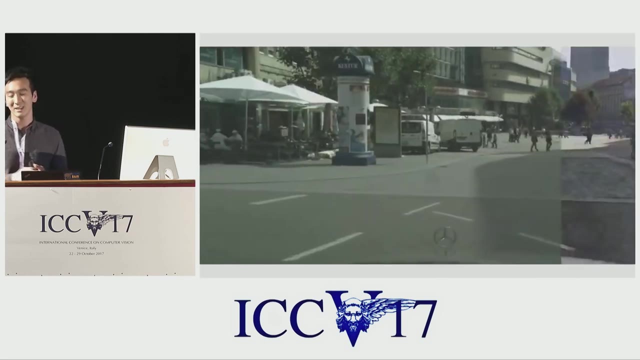 i'm not sure if you can see it clearly, but left side is real and then the right side is fake. uh, this method, uh the the resolution of the image is actually uh 10, uh 1024 by 512, so it's pretty large uh, considering the size of gen. um, so, um, uh. 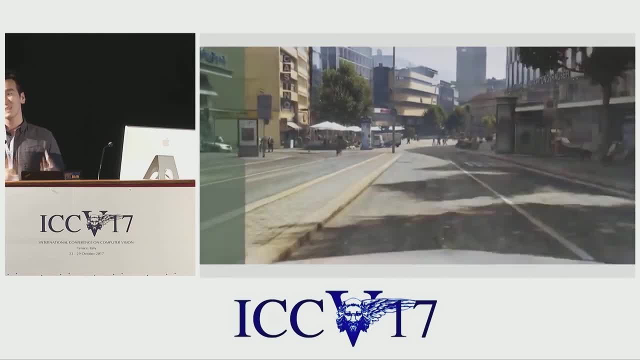 yeah, uh, because cyclogan is fully convolutional, uh, the same architecture can be applied to different resolutions. so the um, the, the resolution of the image i pick. this one is, uh, 10leinberg, an in the architecture you can change it to aportable resolution. so if you look at the dimensions like 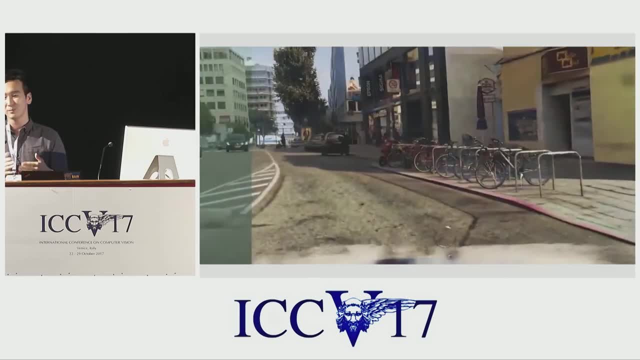 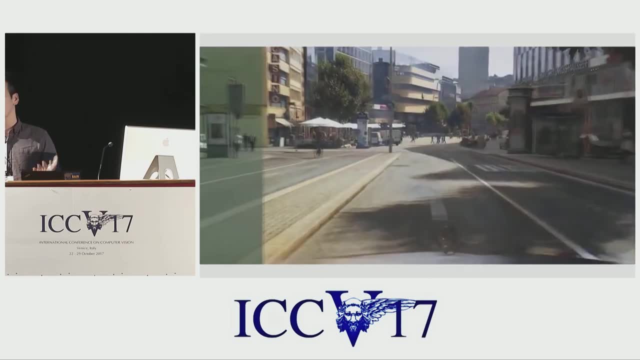 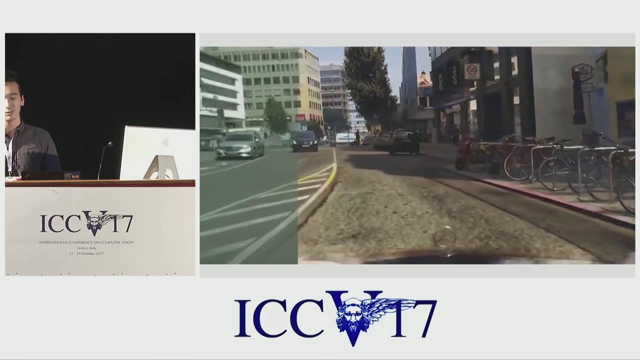 This result was trained using 400 by 400 cropped patches of the original image And then at test time. because we don't have to load the discriminator and then we only need to load one generator in one direction, we can actually run it at much higher resolution. 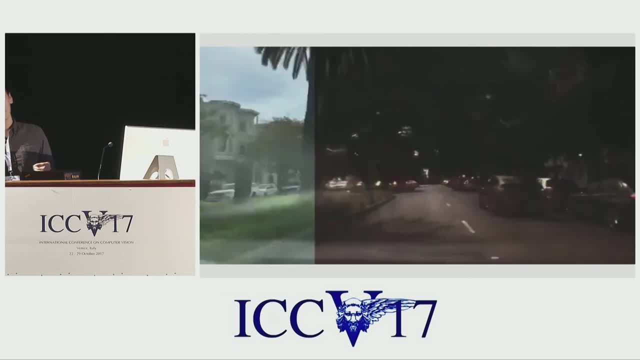 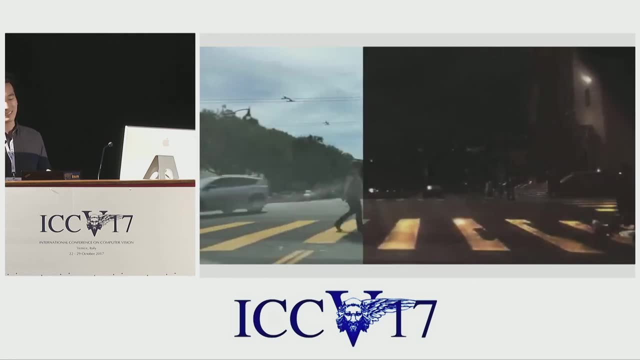 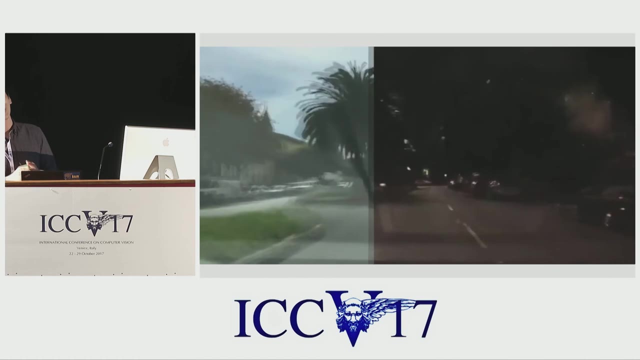 We also ran CycleGAN on day-to-night driving data set. This is for free. There's no- Yes, yeah, We ran this per frame. There's no smoothing between the frames, So it might be a little bit flickering, but it's amazing that we didn't do anything. 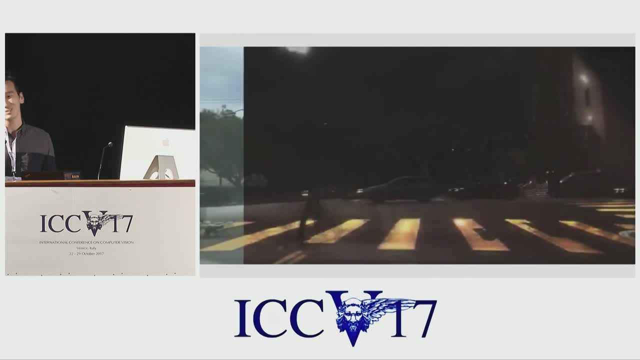 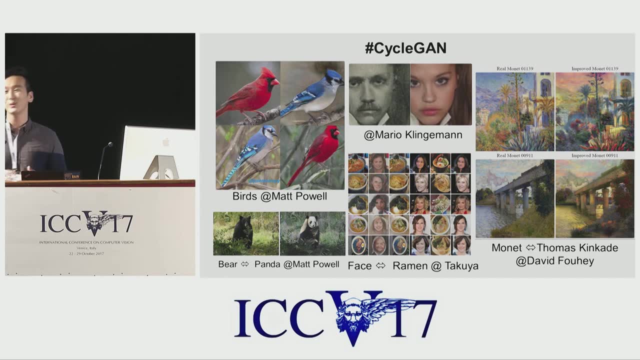 to make it look nice on videos, And it still looks pretty nice. CycleGAN got pretty popular online, So lots of people on Twitter have contributed to different applications of CycleGAN. Here I'm showing some results that looked interesting. My favorite is bottom left. 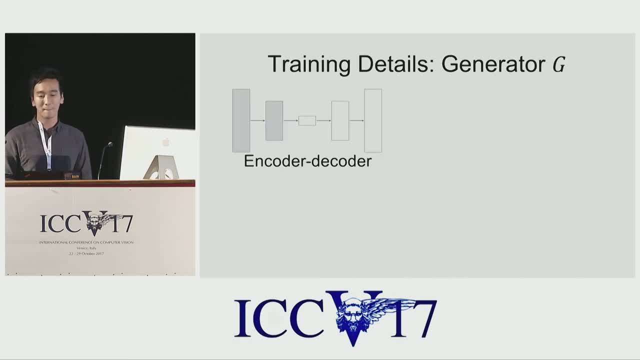 Bear to Pine, Bear to Pine. Let me finish by sharing some implementation details of CycleGAN. So, as talked previously, in Pix2Pix we experimented with encoder decoder like auto-encoder architecture, And then we also experimented with unet architecture. 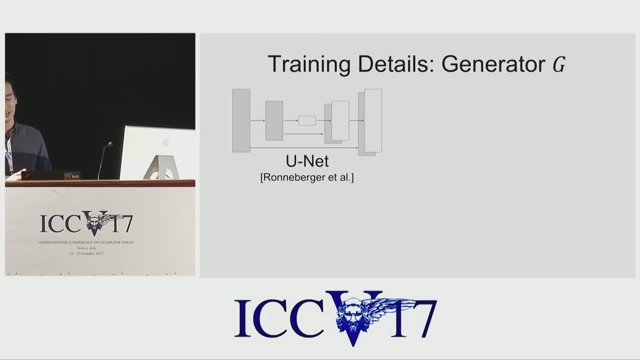 which has skip connections between layers of the architecture. In CycleGAN we switched from the over to resnet, so the idea is the same. the reason that we didn't use encoder, decoder and then use unit instead is because we had skip connections that can. 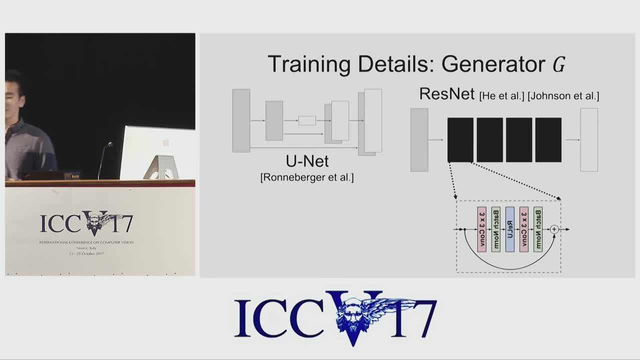 keep the details of the input image. resnet basically have the same skip connections and also it doesn't have bottleneck in the middle, so you can keep the details of the input architecture. and then the reason that we switch to resnet instead of unit is that resnet has fewer parameters, so it it works. 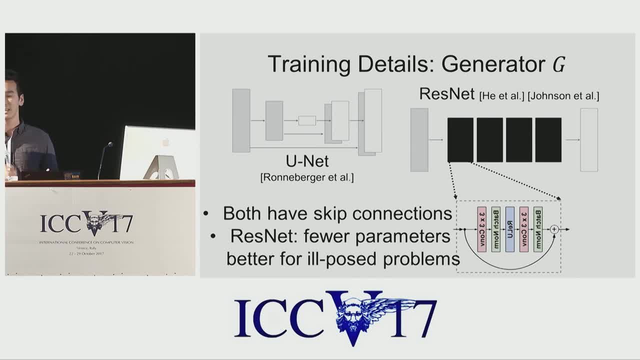 better when the problem is ill-posed, like in case of CycleGAN, we don't have ground truth target image given the input image. so having fewer parameters and also making it fully convolutional, working on working at the patch level instead of the entire image level, makes the training what? much more stable. 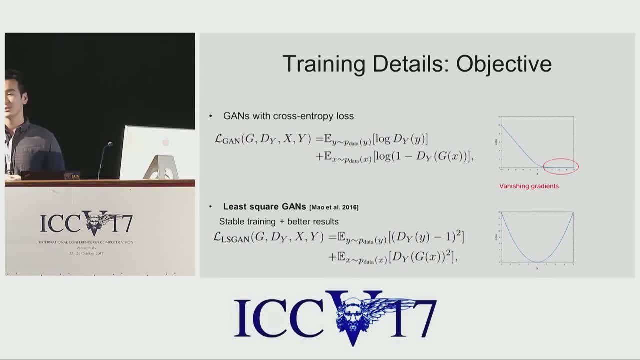 you. instead of our regular- again cross entropy loss objective, we used LSGAN, least square again. the motivation of LSGAN is that the original cross entropy loss has this vanishing gradient problem in the objective function, because the discriminator tends to win a lot and in that case we don't get much. 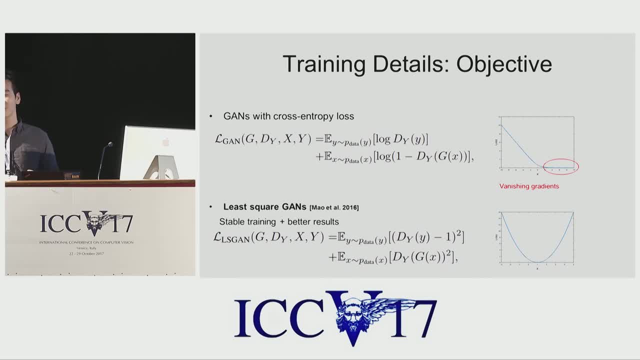 gradient from the discriminator. the motivation of LSGAN is that instead of our cross entropy loss we have a quadratic loss, so we don't have this vanishing gradient problem anymore. so what happens is every night I start a new experiment, happily go to bed, get some good sleep and then tomorrow morning I wake up and then get some. 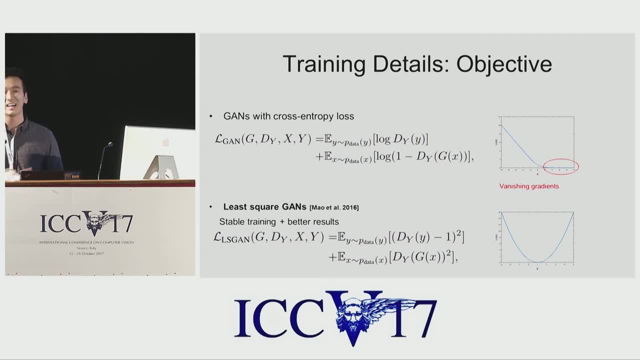 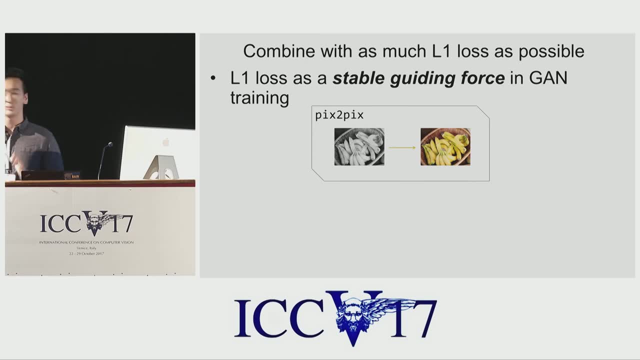 result. that is pretty reasonable. you know, this is an ideal lifestyle of GAN researchers, I think. and lastly, another way to look at CycleGAN is combining: combining, adding as much L1 loss as possible. So in Pix2Pix we combined L1 loss. 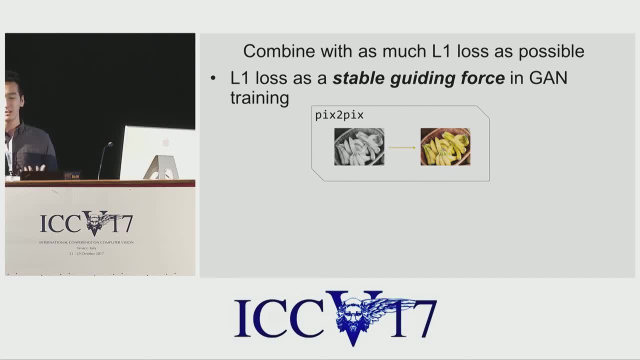 and also GAN loss for better training. So this L1 loss is a fixed target so it stabilizes the training of GAN In CycleGAN. unfortunately we don't have that correspondence anymore, so we couldn't enforce L1 loss. 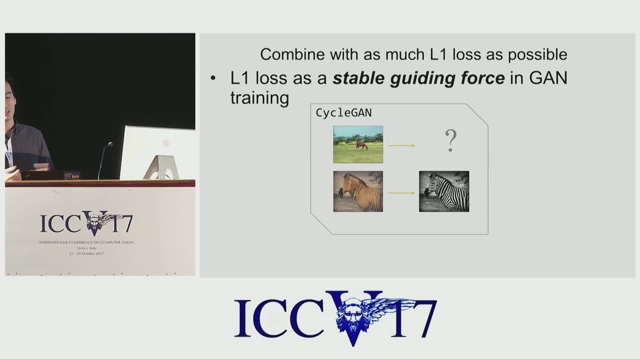 But another way that is less strong, but something that we can still do is, instead of real horse, given fake image of horse. we know the target image. It should be the original zebra image that the inverse generator has translated, So maybe we can go even further. 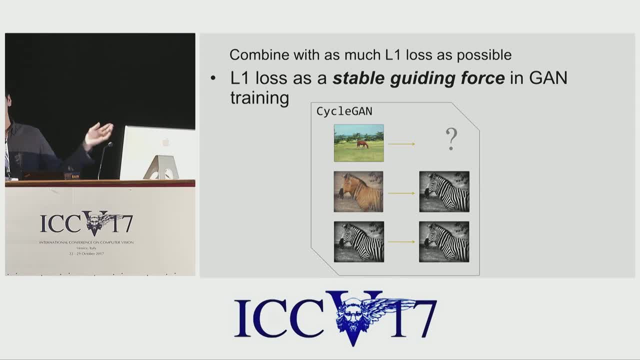 Given an input image as the zebra, which is from the target dataset, what it should do is it shouldn't do anything. So, given an image of zebra, it should do identity mapping. So I just add that as additional loss. 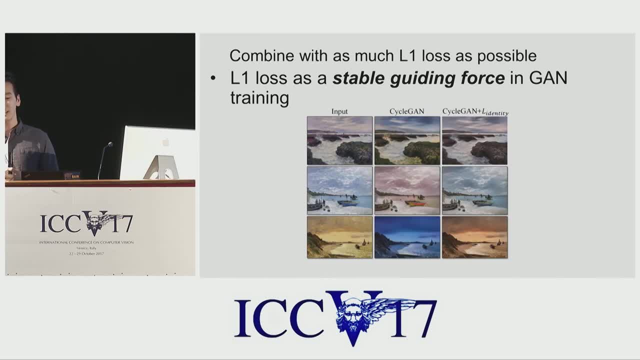 then it seems to help training of CycleGAN. So in some cases it like the result kind of changes each time you train. But sometimes the CycleGAN result flicks the color of the input image. So if you look at the bottom row, 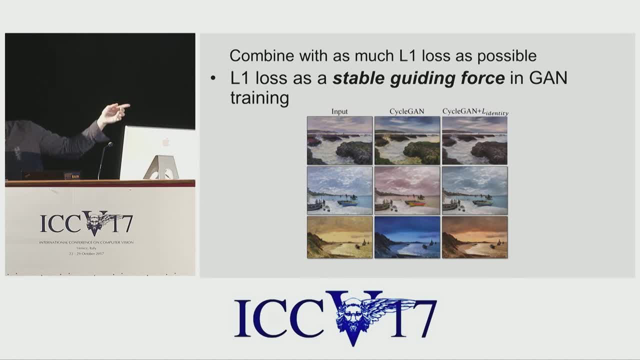 this is Monet's painting of sunset, but you can see that the sun is gone now. It's all bluish. it looks like it's quite after sunset. So in order to prevent that, you have to do a lot of work. 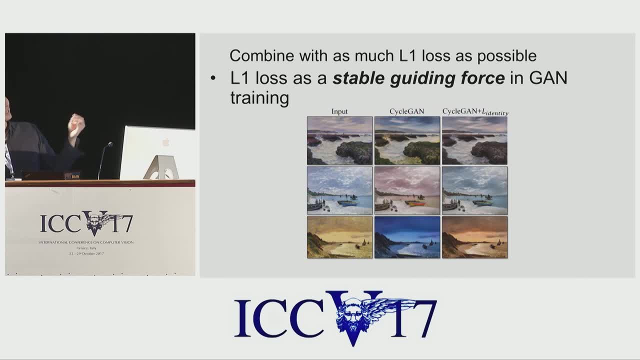 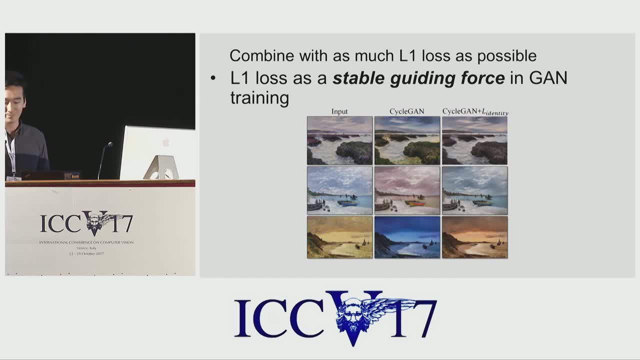 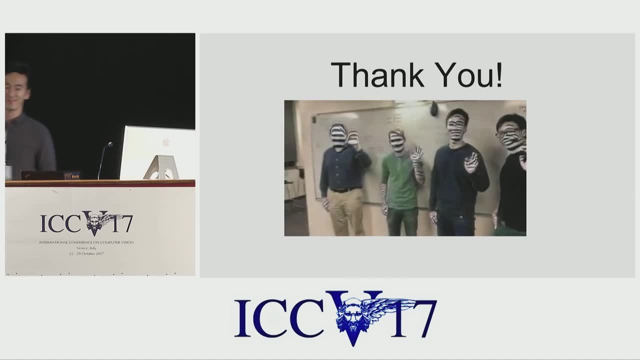 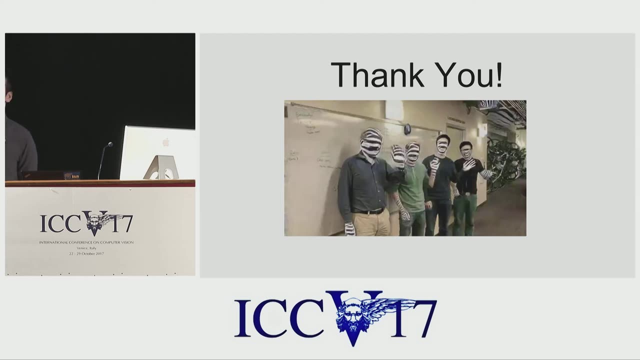 changing the color so much and it's doing something more reasonable. Thank you, I'll take questions, Any questions, for either of us. It's time to go home, I think, alright. so the question from Samjeev is, of course, you know what are we going to do mathematically? What is you know what? if it's not a distribution, then you know what is a way to think about conditional GANs. I think the issue with conditional GANs are is that maybe you can still think of it as kind of a mini distribution, right, given what you're conditioning on, right. 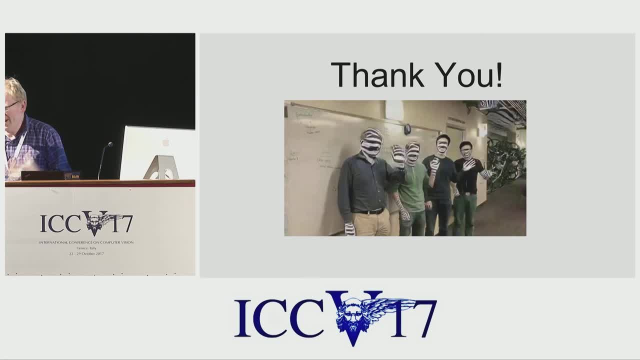 It's still. It's still a distribution, but it's a much more manageable one. So you know, maybe when you can, you know, given like, for example, a grayscale image, then you're already in the right neighborhood. 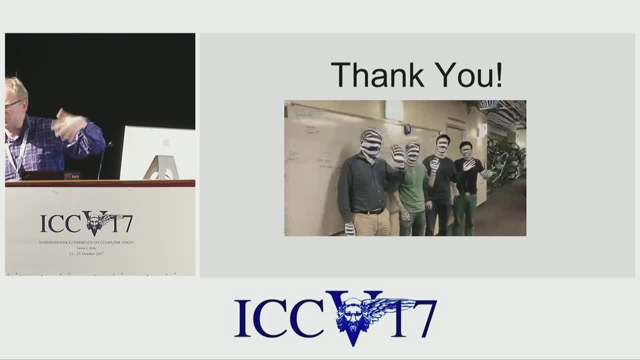 And so you're basically your distribution is: what can you do with that grayscale image as your condition? Maybe it's not that hard, But even then we- you know, multimodality is still a problem, You know- can we generate, you know, multiple colorization of the same grayscale image. 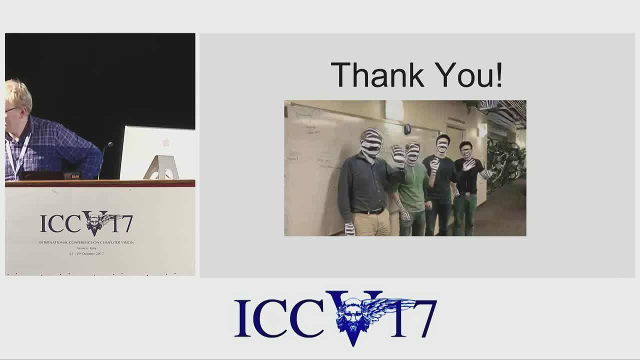 Not really Not easily. It's still. you know there's a bunch of papers coming out, but it's not a solved problem. I think you know it's as long as we have something that can produce, you know, can take whatever goal you have and project it onto the manifold. 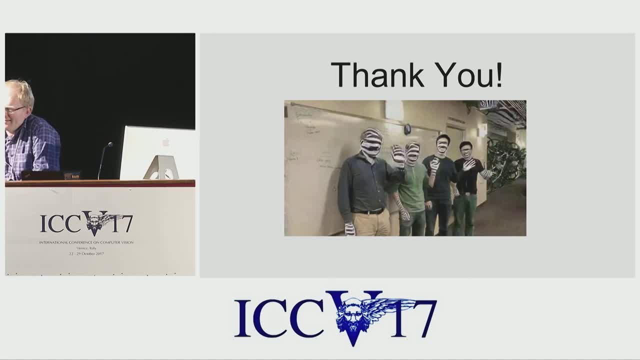 Of natural images. I think that's a cool enough, at least for you know, for graphics people that's already a really exciting thing, And there we don't really care about a distribution. you know how much of the natural image manifold, are you? 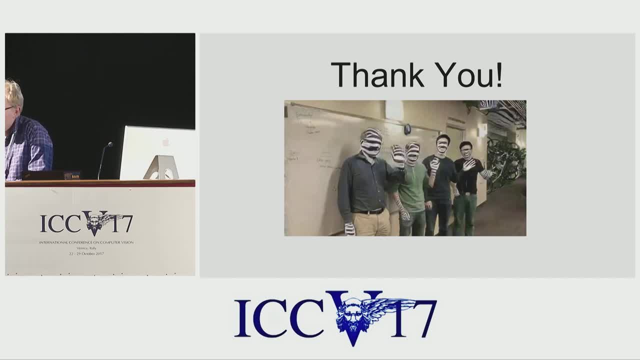 So I think that's the exciting thing for us And you know, I'm- yeah, I'm not quite sure it's really the whole, The whole, you know, generative side of story maybe is not that relevant, at least for some problems. 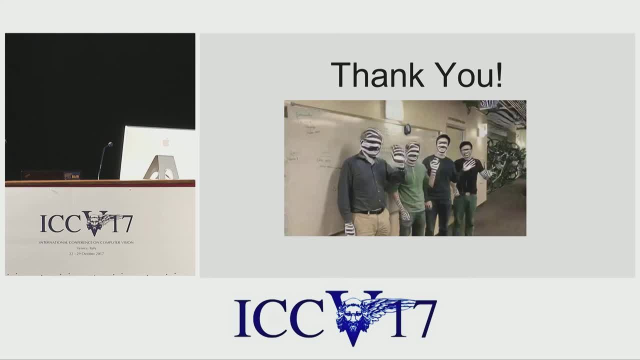 Yeah, Hey, thanks for the presentation. So I want to ask about the phenomenon. I'm over here, No, Hi. So I want to ask about the phenomenon about like sort of skin turning into zebra. So like you sort of gave the rationale that, like you know, you haven't trained on sort of humans. 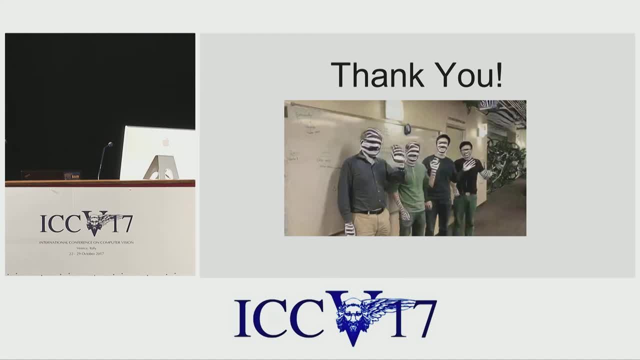 So it doesn't really matter. You don't really know what to do. But you could also say the same thing about like, about, like you know, sort of indoor scenes in general. So I'm sort of wondering if you have any explanation for, like you know, why the clothes or like the whiteboard in this image aren't turning into zebras as well. 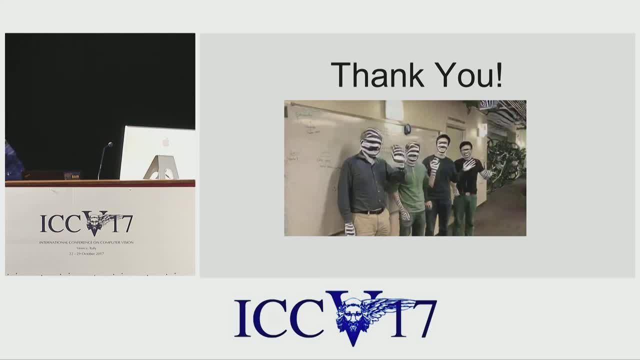 Is there something special about, like skin that might be causing that? Well, we can, yeah, we can- see what my feeling? Yeah, So you know why is it focusing on the skin and not on the clothes? It's basically, it was trained. 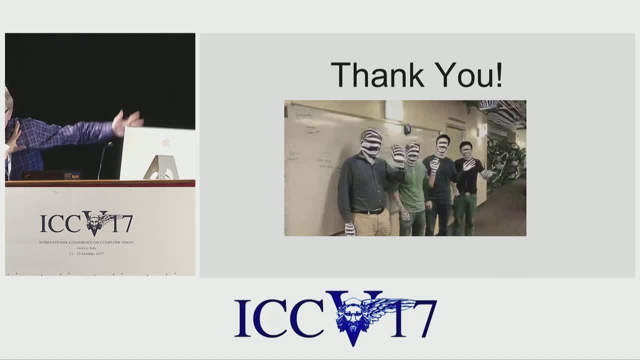 It was trained on on on horses In in like in outdoors, Right? So I suspect that it's basically trying to solve a binary factorization. You know, are you a horse or are you a background, Right? Are you something that is zebraable or you're something that's not zebraable? 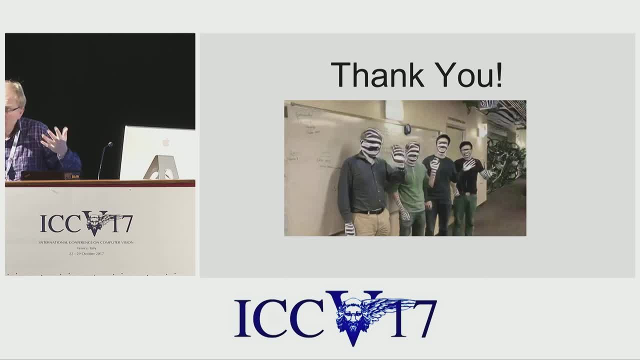 And you know, for one reason or another it thought that skin, you know leather, right, it is more like a horse skin than than other things. So we have seen, I think, in the demos earlier, that people with it, with some type of clothes, have been zebrafied, but other type not. 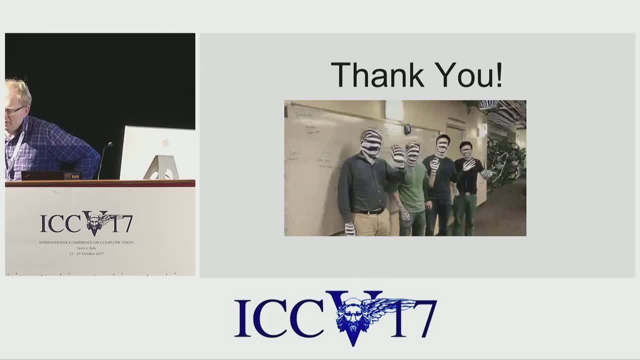 So I think it's suspect. it's basically: you know how close you are to looking like a horse. Do you have any anything to add? I think it really depends on which training data set you used, because, CycleGAN- the networks are picking up on the biases in the data set. 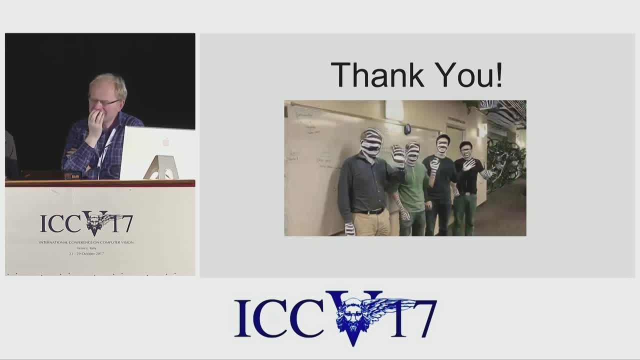 And I think the horse data set that I trained on was from ImageNet. It's category wild horse. So I think it picks up on color a lot, because oftentimes the horse is standing on top of grass, which is usually green, So I think there is like a very strong hint just by looking at color. 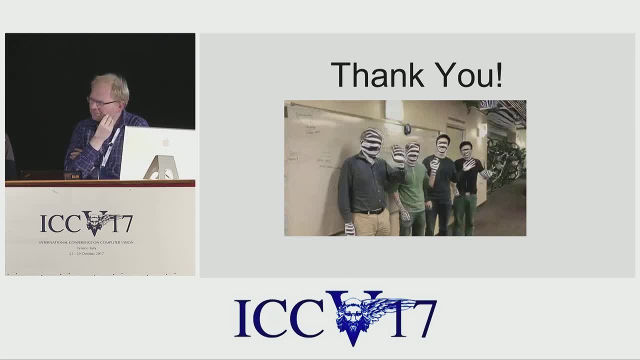 And then human face has a similar color as horse. So I think that's why sometimes, All right, Thanks, All right. The question is: do you think GANs can be competitive in a traditional computer vision problem like sigmatic segmentation? 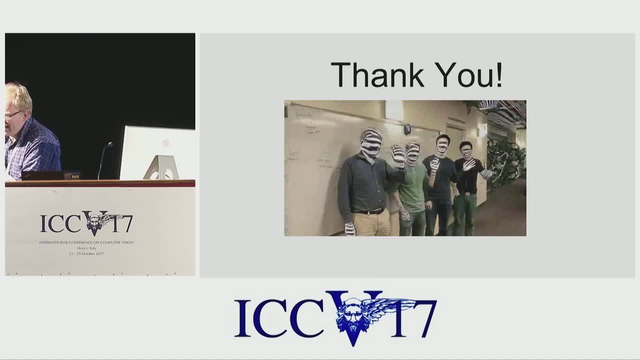 We haven't been able to get competitive results with. you know, with Pix2Pix, for example, It can do semantic segmentation, just very simple. Just, you know, throw in the, The task, that just does something and it does reasonable things, but it's, it's not competitive to the specially specially engineered efforts. 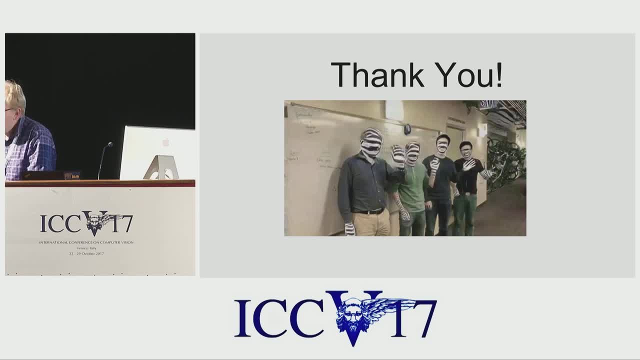 I think at this point, you know, if you have a very, you know, if you have a smart grad student and you tell them to write a tailor made, you know, horse to zebra translator, that would also be better than CycleGAN, right. 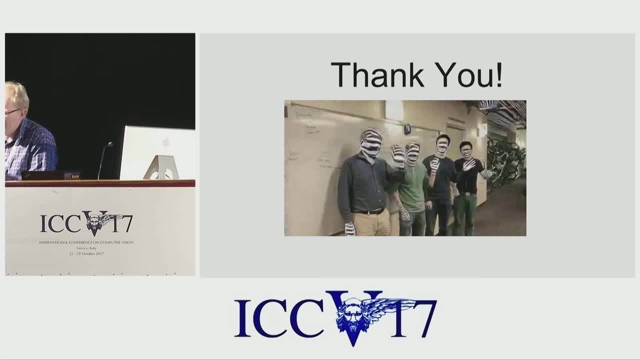 I think any time you want to do something that's problem specific, You should be able to do better. So I think you know for any particular task you're doing- you know self-driving car or something- the first thing to do is to just try to attack the problem directly. 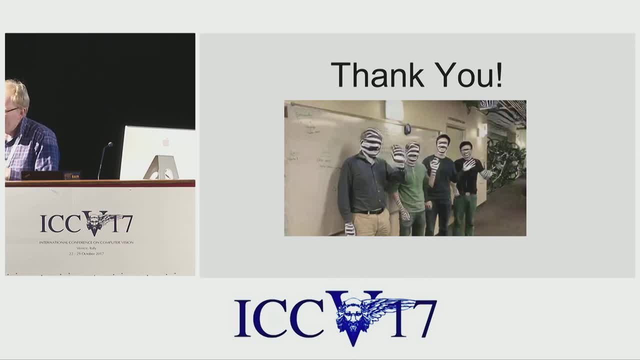 I think the power of GANs is the generality, And I think that's the exciting thing. So so I think, yeah, I think that that that's the, that's the stuff, that's that's going to give you a win. that it's, you know, given a new task, you know, transferring to a new scenario. 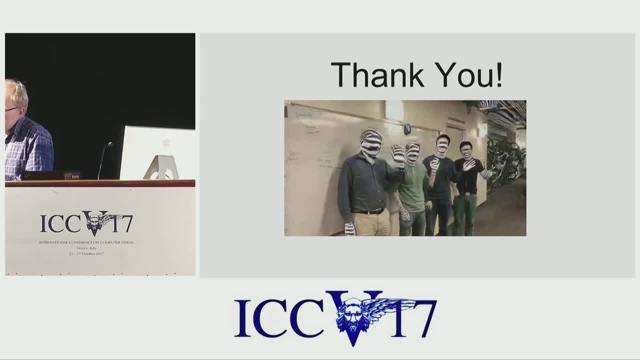 It, it's likely to to do something much more reasonable than whatever your hand handcrafted thing is. the same way, as you know, semantic segmentation are, you know, approaches haven't really been able to transfer that well to, to other things you know, without a lot of hacking. 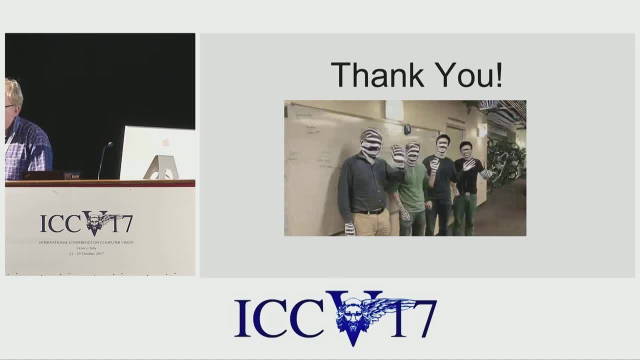 And this at least promises to be just very transferable without any parameter tuning at all. I have a question. Yeah, So at the end you talked a little bit about the color sometimes flipping, And so the identity mapping helps that. But there's kind of a more general problem that any like permutation in the other space. there's no constraint preventing that. 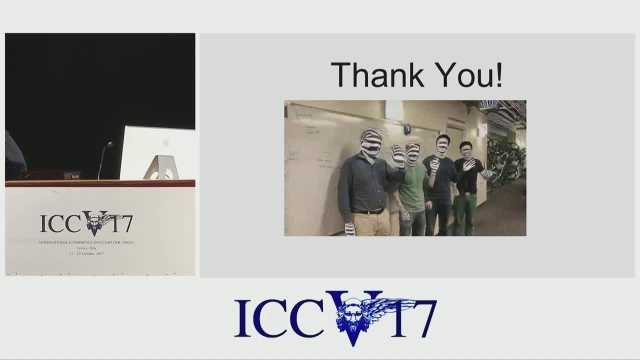 And the identity kind of helps that, but it doesn't actually enforce that. Do you have thoughts on how you would? So I think we are relying on common sense in a sense. So we are doing this optimization in GAN training, and then the easiest solution should be the one that's easiest to translate, which is the most reasonable translation to human beings, but sometimes that's not the case. 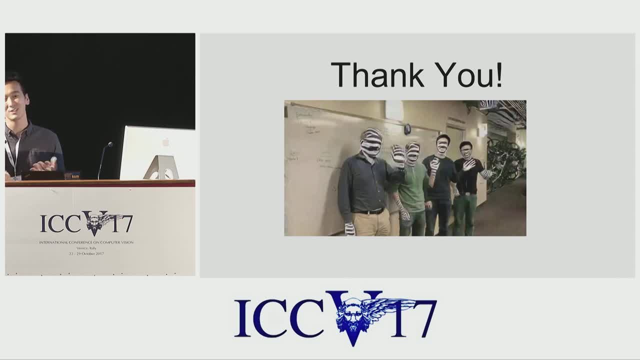 That's why we edit the identity loss or even change the generator architecture, but more or less we're surprised to see that. you know, even though we have many, many permutations that are possible for CycleGAN to do, it ends up with something that we can't do. 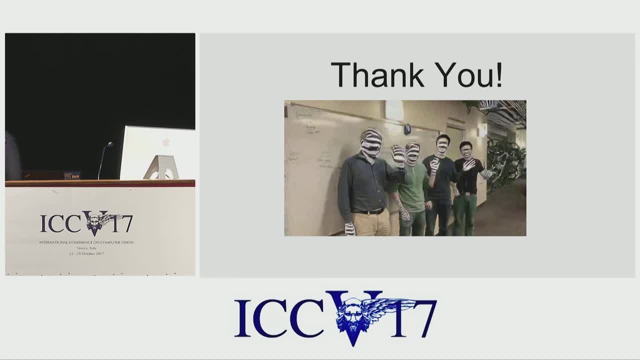 Yeah, I think this is a kind of a more fundamental issue that you know there is. there is a way, a lot of ways, for this thing to cheat, But somehow, for some reason, it cheats much less often than we expected. 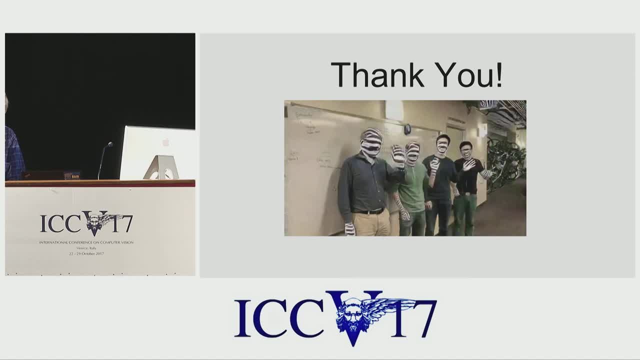 And I think we still don't quite know why this is. It could be just an artifact of, you know, the architecture, like the convolutional architectures. maybe Somehow steer you away from the really nasty solutions, Because really the problem is crazily under-constrained, even with the cycles right.